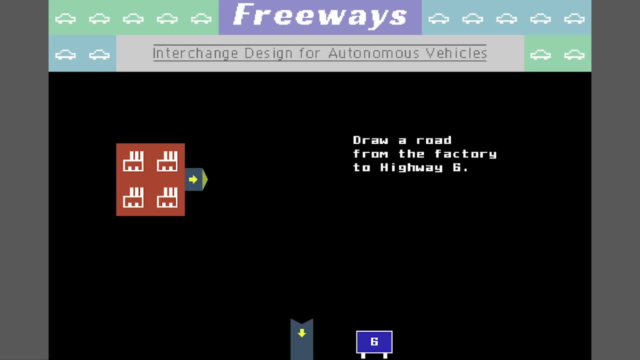 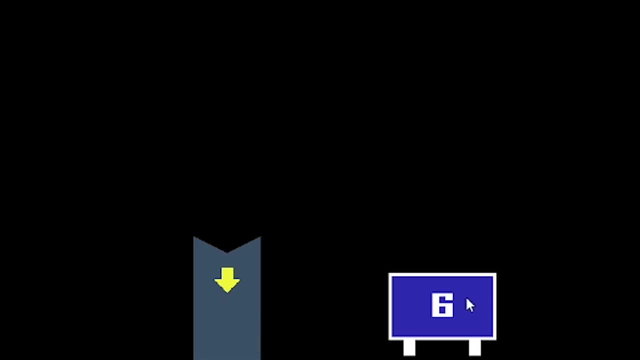 years, But I'm actually super excited to play this. So, basically, we just do what the game says. The game says: draw a road from the factory to highway 6.. So you can see there's a little sign 6 there and this is our factory. So we've got. we've even got arrows to help us. Basically, you. 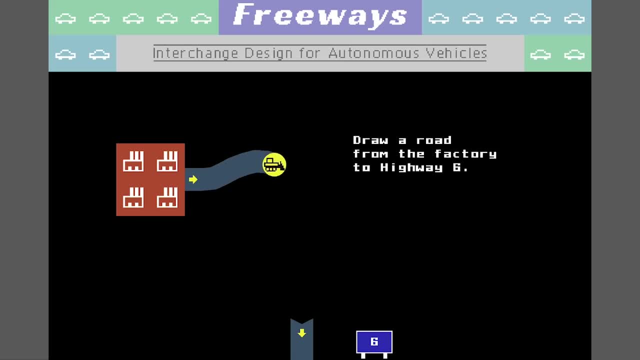 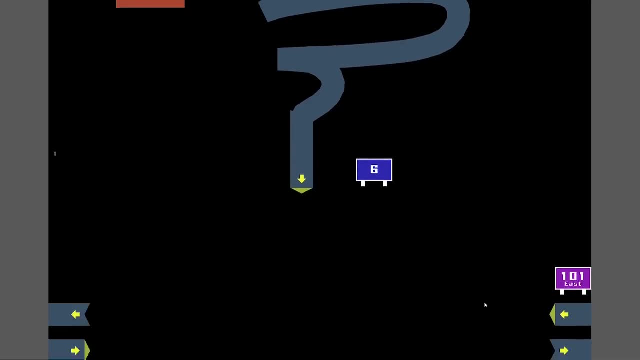 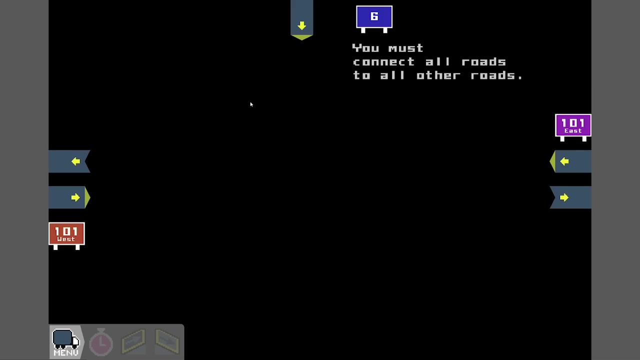 click on that and then you can start drawing whatever you want. So you can literally just like: Yes, Yes, I love this game. I love this game already, Right, but this is where it gets a little bit more complicated. We've got, like we've got- three arms. So on the left and right we've got. 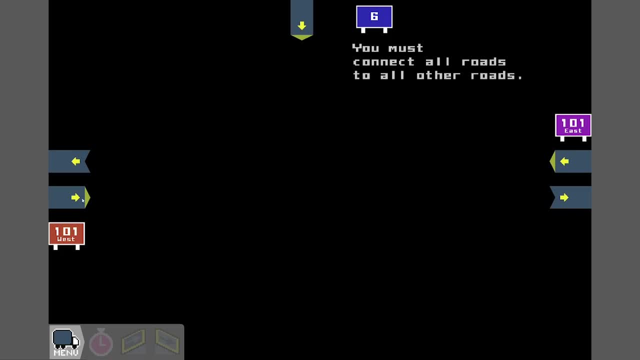 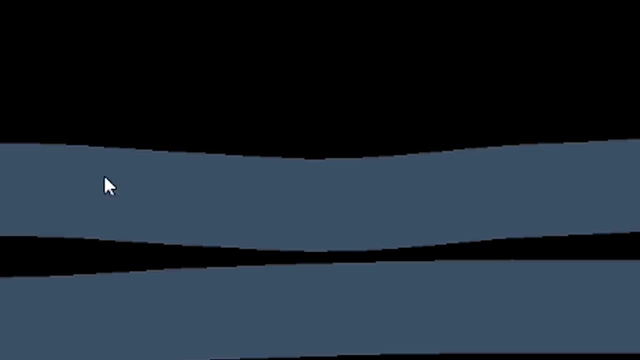 in and out roads and then down the top. we've just got an in road. So, as with most highways, I'm going to start off with just the straight dual carriageway- Not the straightest dual carriageway you'll ever see- And then, as it says here, click highway signs. 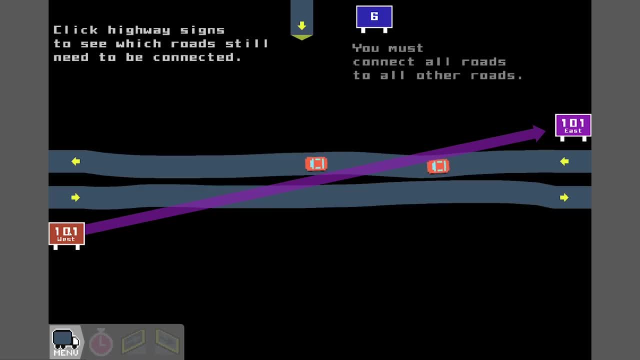 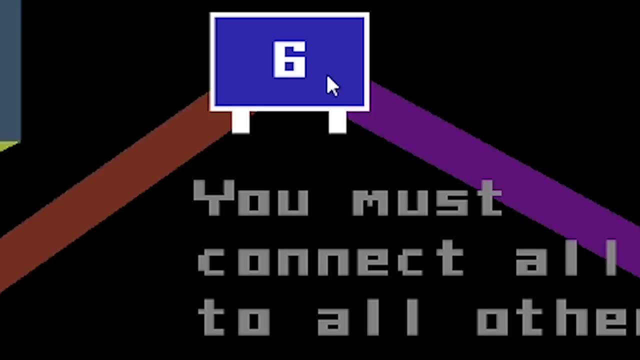 to see which roads still need to be connected. So if we click on here, you can see we've just got to go straight to purple and we've done that. Likewise, if we click on the purple sign, we've just got a red arrow to the red sign, But if we click on this one, you can see we've got to go both ways. 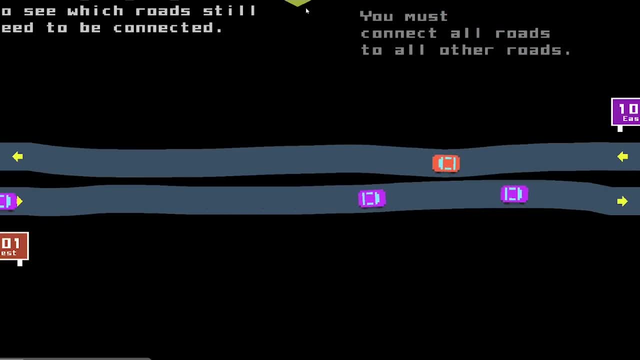 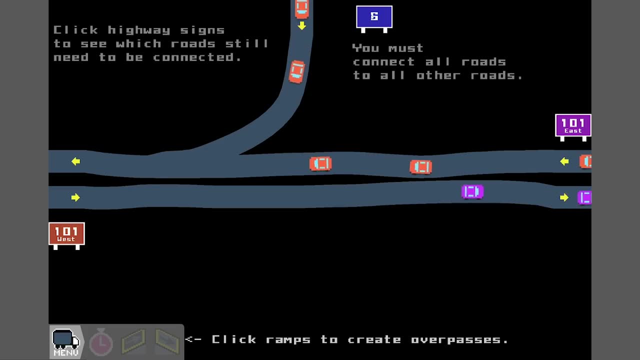 and they're flashing. Flashing means you haven't completed a suitable route, So the first one will just a nice bend like that. And now when you click on this, you can see only the purple one's flashing. So to do that one, we're going to just do a slip route off. But notice down here, click. 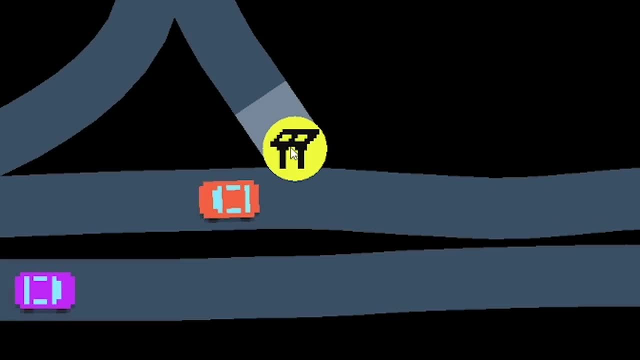 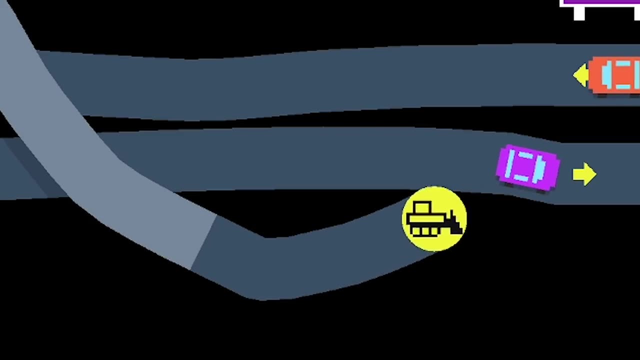 ramps to create overpasses. We can go like up, and now we're like slightly higher, Then we can come across and then press the down ramp again And now we've made like a little bridge And when we just connect in, like that network complete. So you can see now the traffic can now complete journey in. 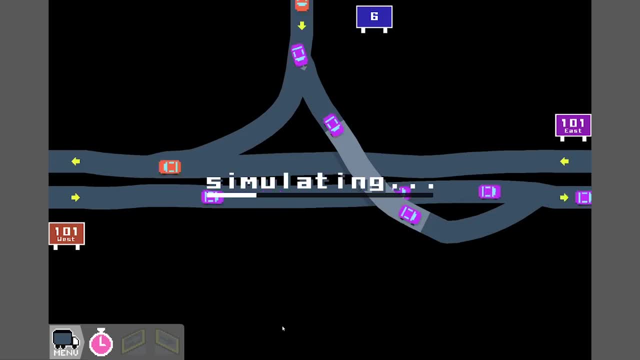 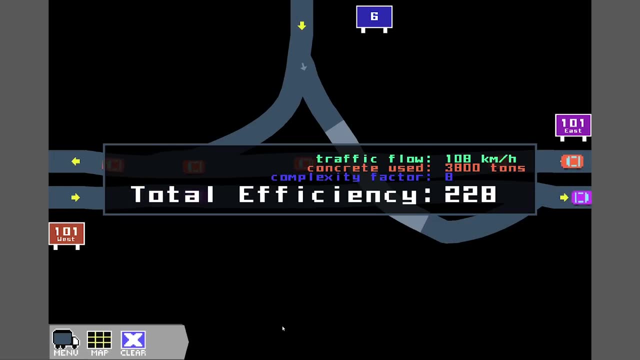 all directions. So if we press this stopwatch button, this like simulates, like loads of traffic over time. The aim of the game is to make sure you can get to the end. If you have too much traffic, if it's not like fluid enough, then it will tell you that and you have to retry. We can see. 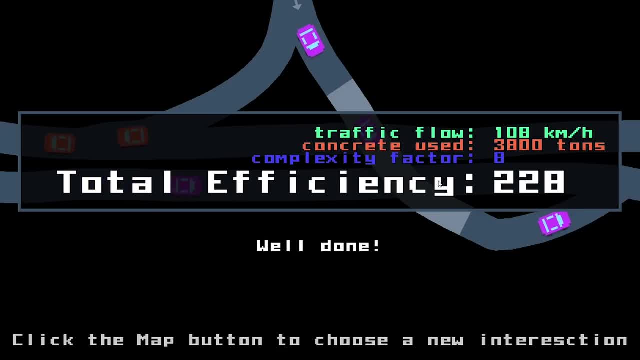 here. it gives you like a load of different stuff and like a total efficiency score 228.. Not really sure if that's any good. I don't think there's leaderboards or anything on this, But that is quite handy for if we want to compare like different designs- I do- I do feel like we want to. 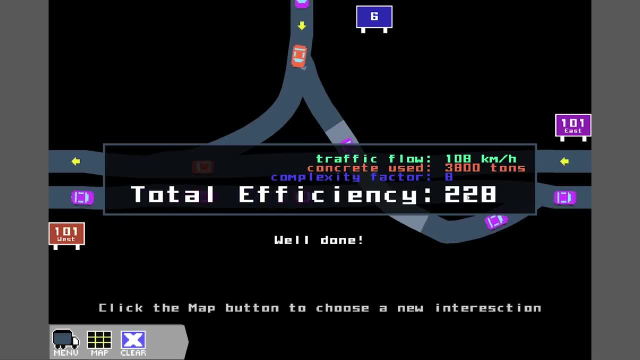 go through. maybe not this video, maybe another video, Maybe like comparing, like proper big layouts. Let me know if you want to see that, But for now we're just gonna sort of wing it and just do whatever comes to my head first, Which will probably be a knob, But now the level is complete. 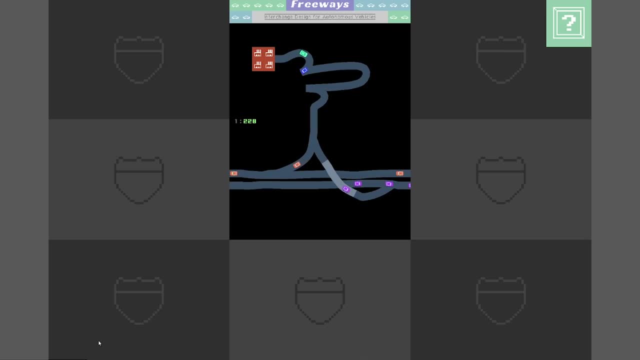 we can come down here and click on map, And that takes us to this. You can see my previous two levels. They're all completed now And they sort of stay there. So all these other tiles, you can click on them and that's another level. So, for example, if we go here, this is next to the level. 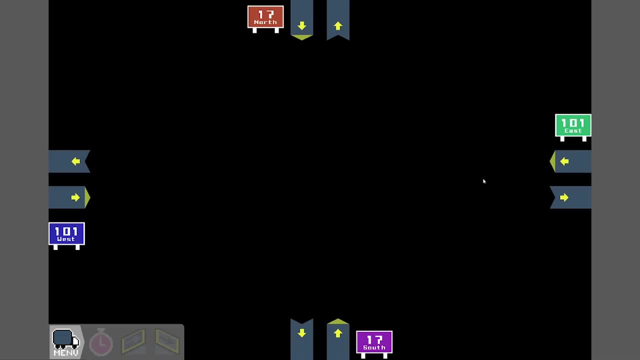 we just did And we've got like a classic four-way junction required And I feel like with this layout we can choose. I'm gonna go with the clover leaf interchange, So essentially I'm gonna do my straight throughs. So there's one And there's the other one. Ideally it was a bit straighter. 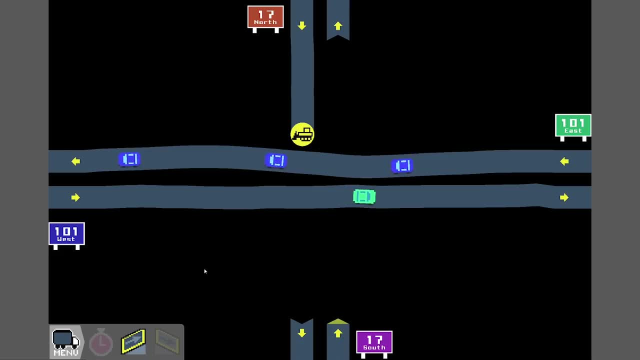 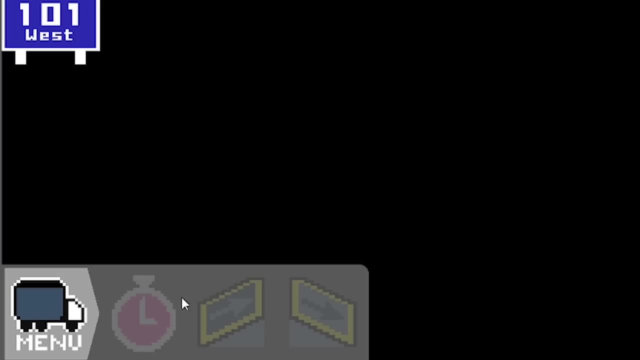 There's no undo in this game, Which is a bit of a shame, if I'm honest. We can go to there and then we can go up, Come across And then back down And basically, if I were to not use this overpass, 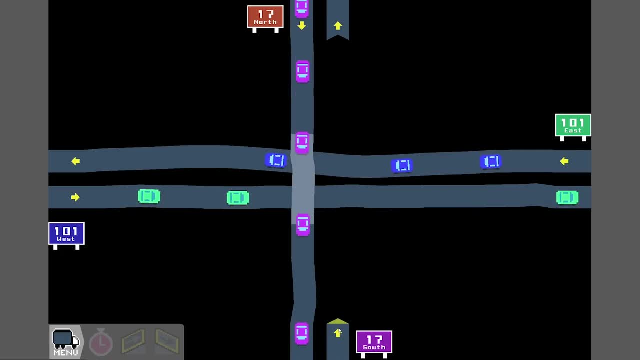 sort of thing We'll just make like a junction, Like a crossroads And, as we know from mini motorways, that's no good for traffic. So this one we can't there Go up, Come across And then back down Nice. So now we've satisfied all the straight through journeys. But obviously we need to do like 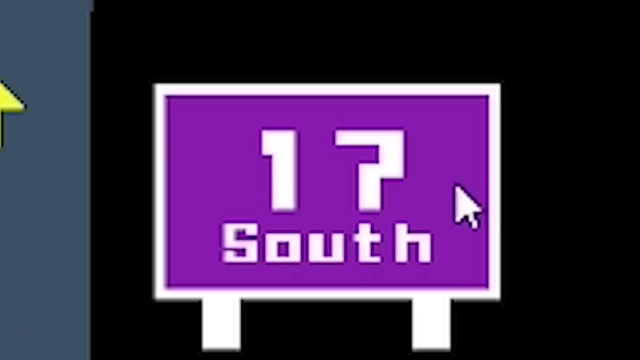 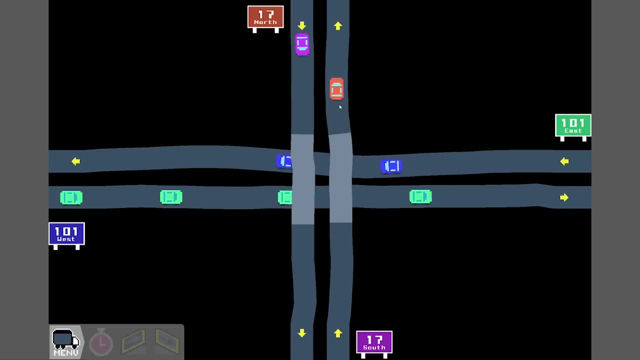 all the corner ones. So for example, these purple people coming from south 17. They're coming up here But they want to go to 101 west. So the way a clover leaf works is you cross over And then from about here you do like a pretty steep curve Like that. So now we should see when someone 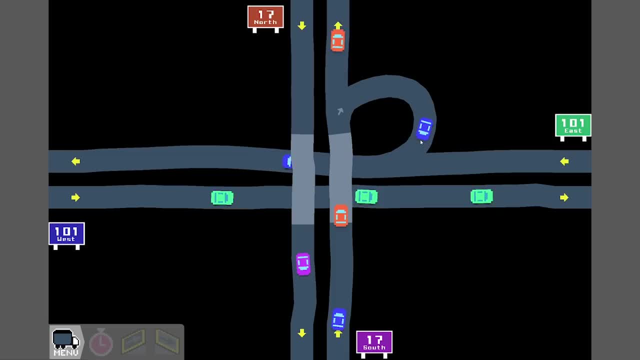 decides they want to go that way. There you go, This blue car, Can you see he's coming around? And then he goes under the bridge that he's just come over, If we just do this for the other direction. So we'll bung one in there. We'll bung one in there. 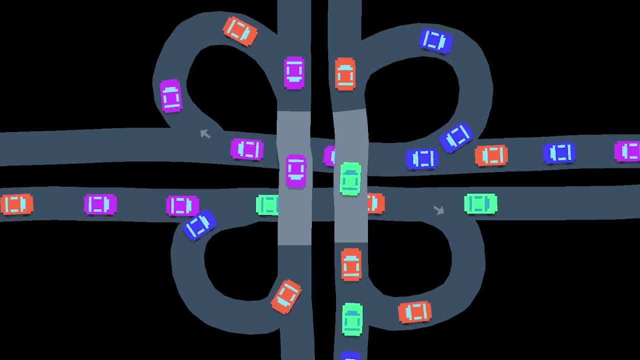 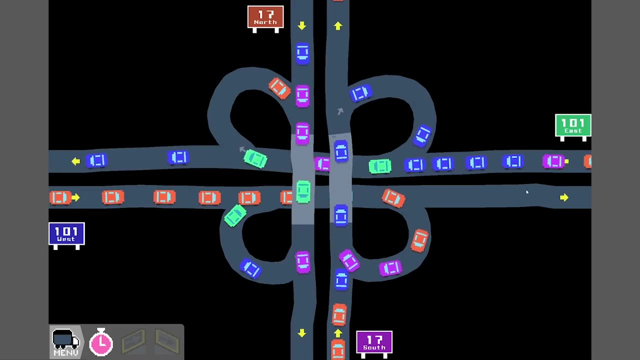 And we'll bung one in there. Now you can see we've completed it. However, you will notice it's a bit of carnage, Because people, for example, if they want to come from the bottom And if they want to go right, They're currently going around the entire thing. So we're actually going to add some. 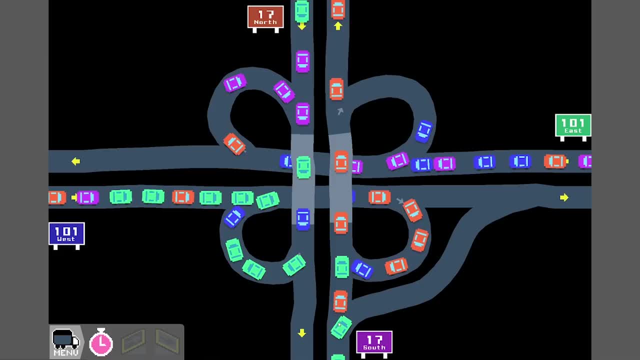 extra roads. You'll see now if we come around here And do that. Now these people, like this green car is doing, They can just get around there nice and easy. I'm going to do this one next, Because this looks like carnage. 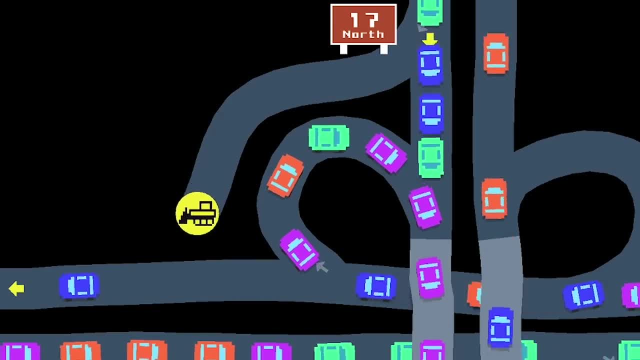 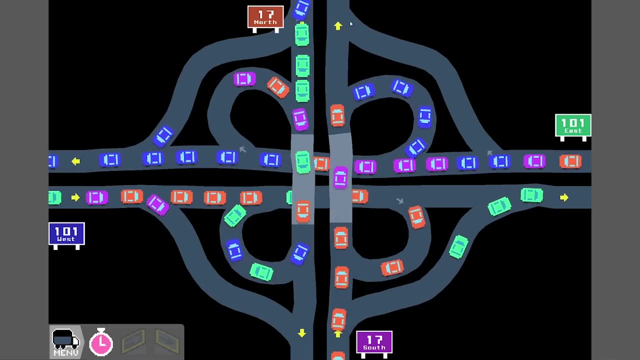 There we go, And then I'll do this one, And then I'll do this one. Right, and you should see in a bit the traffic will sort of get a bit better as people start using these extra arms. Now, hopefully, I've built that one in the right place. No one seems to be turning off There, you. 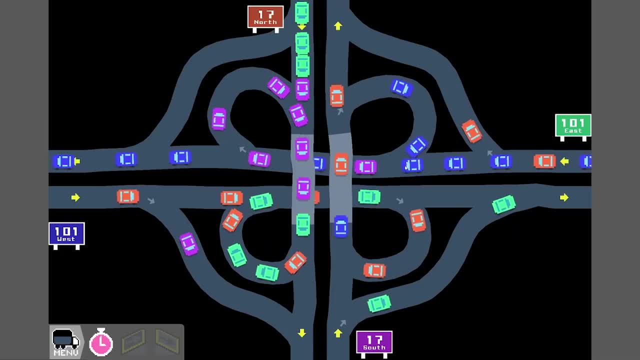 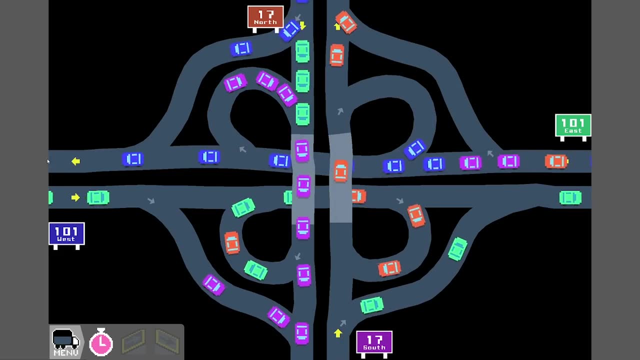 go Orange car. Good orange car. I think the way this works actually, The different colored cars are heading for, like the different signs. So all the orange cars are heading north, All the blue cars are going west, Etc. etc. Now so these clover leaf interchanges, They're not like the best for. 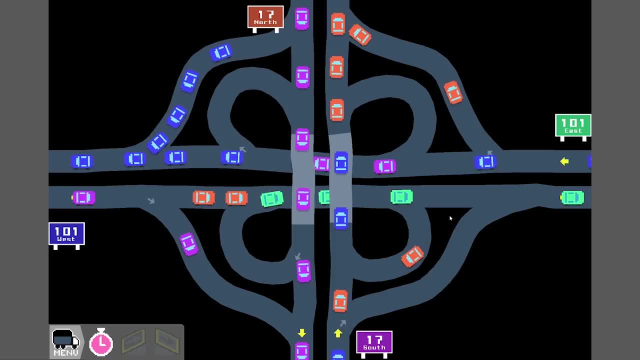 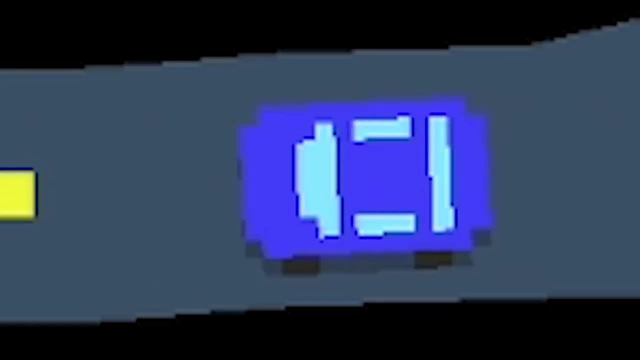 traffic, But they're very good at being cheap. When you build a road, the bridges are the most expensive thing ever. If you think about a road just on the ground, It's literally just road Like the ground. supporting it Still costs a fair bit, But it doesn't cost that much If you then try and 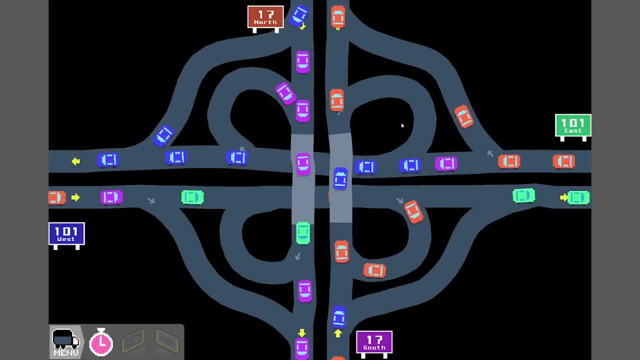 launch that in the air above a road. Think about, like, how much strength and how much material is going to be needed to hold that road in place, And then look at this design. We're satisfying all these different maneuvers. We've only got two very short little bridges in the middle, So that's. 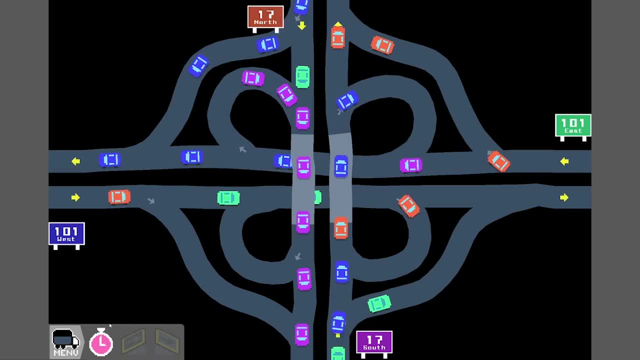 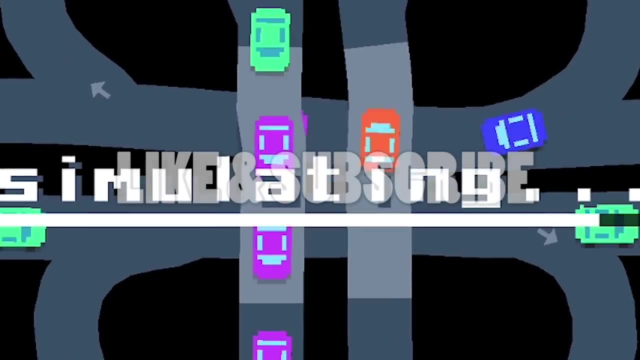 generally why we use the clover leaf interchanges. And now this is all sort of set up: We can press the stopwatch button And it gets simulated. And oh, I thought I was trying to like hypnotize me into like a secret message. But yeah, that's. 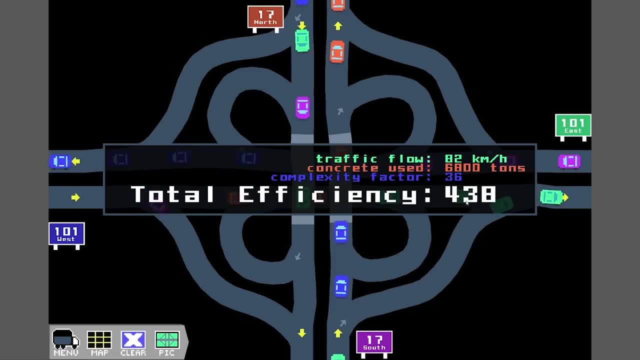 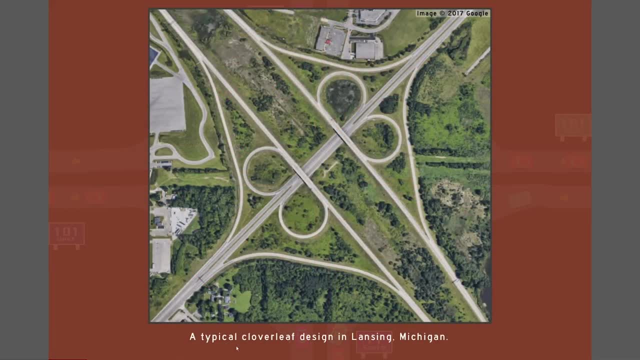 that's bloody efficient compared to my- uh, my last level, That's 438. we got there. Now we've also gained this Pick. I don't know what that means, I assume. take a picture of it. Oh look, it shows you what I've designed The game knows. Yeah, so that's. that's a real life. typical clover leaf. 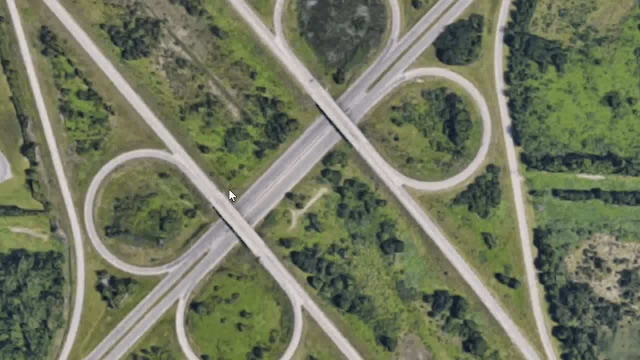 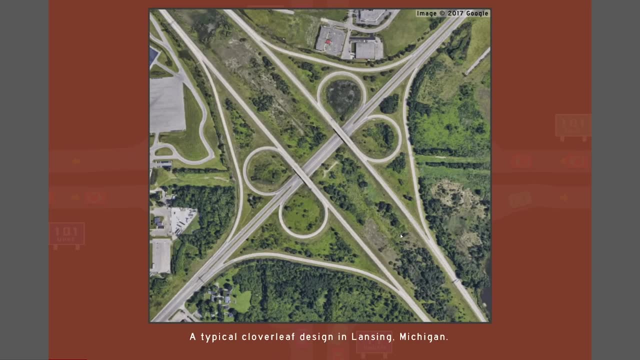 design. Oh, this is cool. I'm going to try and get all the different ones. We can see there's only two little bridges there, Like one there and one there. All the rest is at grade. we call it All at ground level. So nice and cheap. Sweet, This game's wicked. 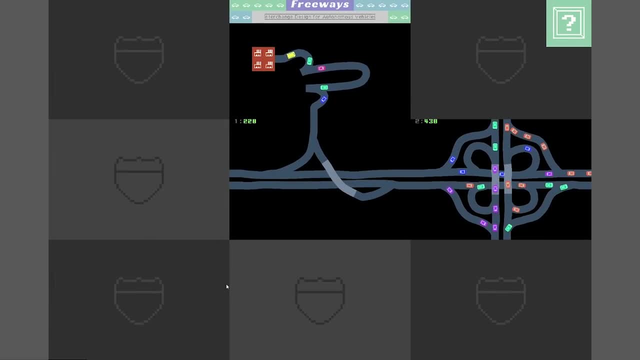 I am loving this. All right, so we can go, We can click on map And we're back to the map. I love that, like it keeps all your levels. They're all intermingled. I think once you like fill in the square, it then expands, So it's not just nine levels. There's a lot to this, So shall we go in. 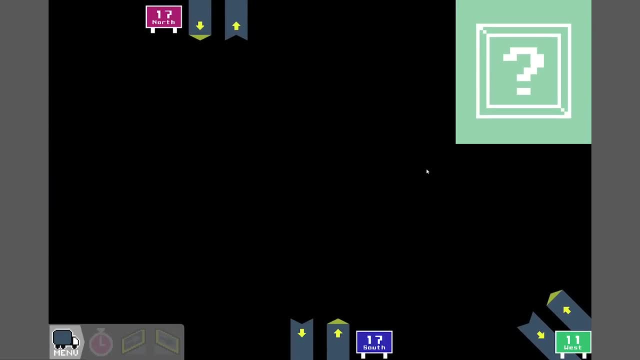 the top right. Yeah, let's go In the top right. What have we got up here? Oh, we got like a three-way sort of. We got like a straight up and then a little sneaky one on the right. All right, so for this one we're just gonna. 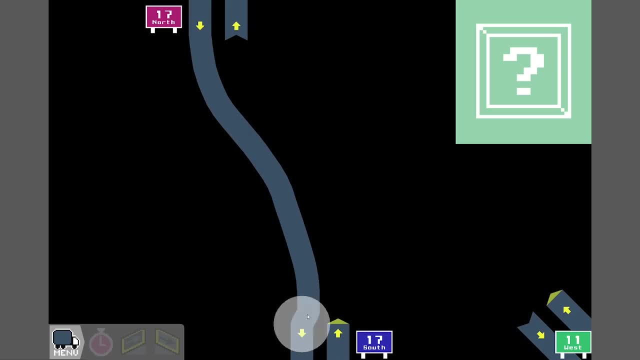 we're just gonna see what happens. I'm not gonna do any real highway stuff. We're gonna- Oh, that's a bit of a dodgy turn. We're gonna just keep this as like a normal sort of s-bend. We're gonna do. 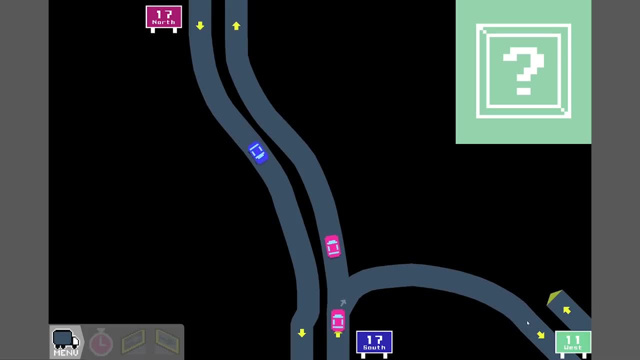 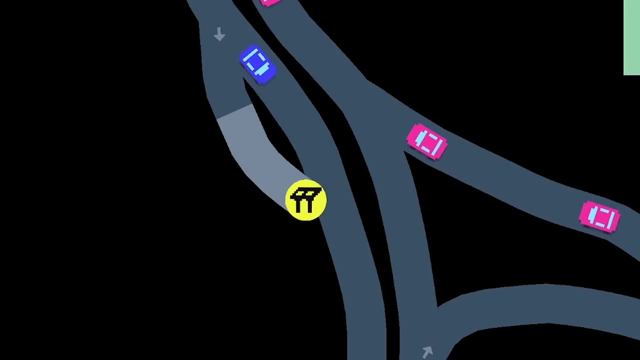 we're gonna do from blue down to green. So I'm just gonna do like a right hand turn, like that We've got to go from green to pink. So I guess we'll just go up and sort of join there. Now we pink to green. So I'm thinking if we come off like there, we can go up over these two and then 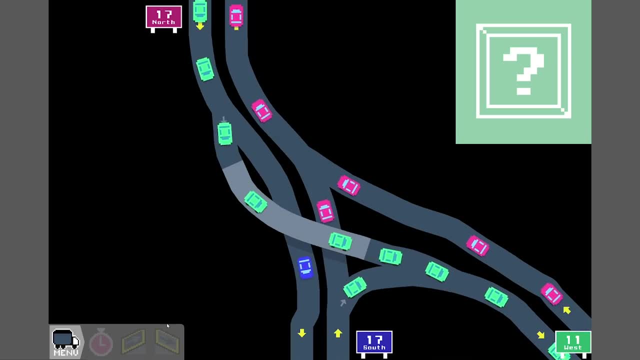 straight down and connect in there like that. I think this is a good opportunity to show you the ramps. They can actually go up another level. So if we were to come off here, Start heading that direction, Then we can ramp up, Come across here And then when we get to that, we can actually ramp. 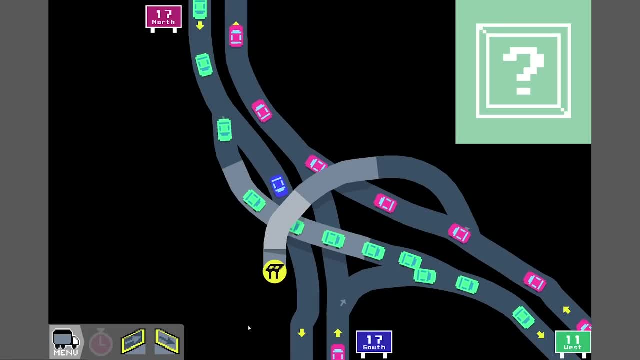 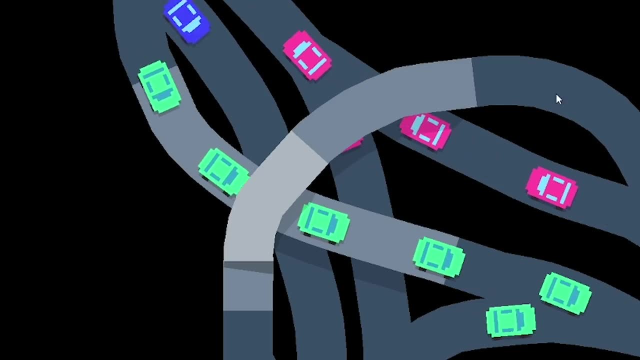 up again. So now you can see we're like over the top of that And then down And then down And then just connect back in Network complete. So you can see this one It's like a light blue, Lighter shade of grey, So we should be able to follow the blue cars now. So he's down And then 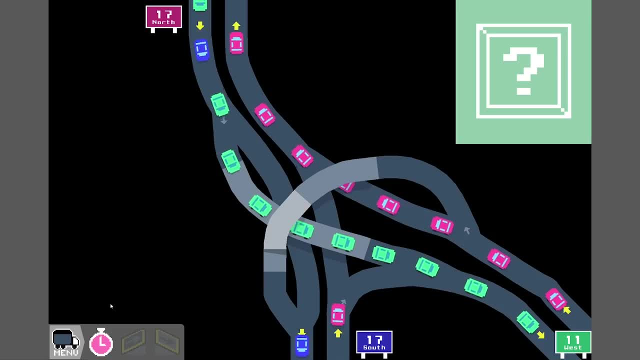 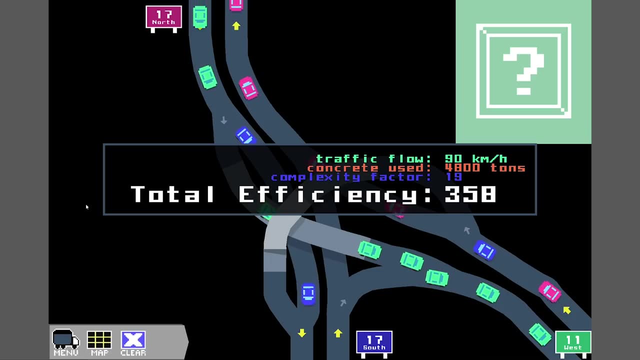 he's. he's gone up, He's gone up again And then down. Cool Right, Let's press the stopwatch button and simulate this bad boy. That's a lot of traffic. Nice Efficiency: 358.. Again, we're showing some sort of leaderboard, just so I could see if I was doing good or not. But right, So do. 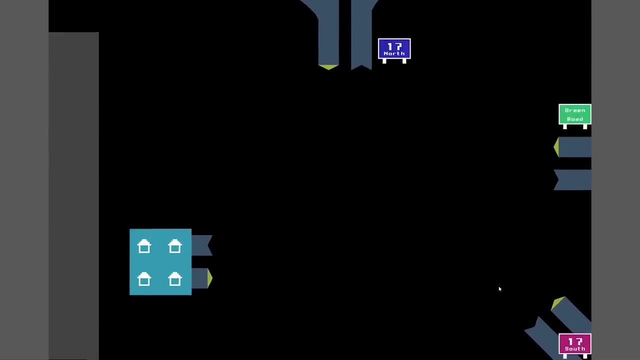 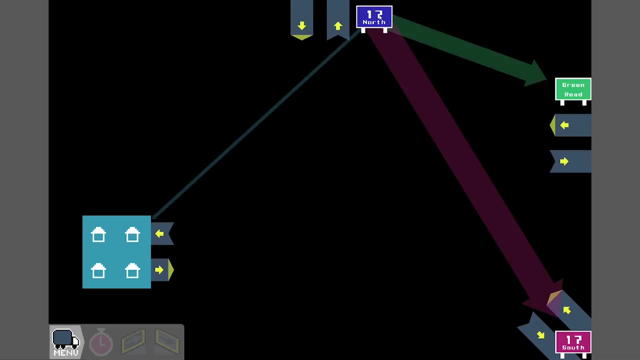 we go. Let's go underneath our cloverleaf design. Oh, we've got another like four way up. It's a bit staggered. The other thing to like take note of on this game: When you click on these signs, can you see the arrows are different thicknesses, So that's sort of where the 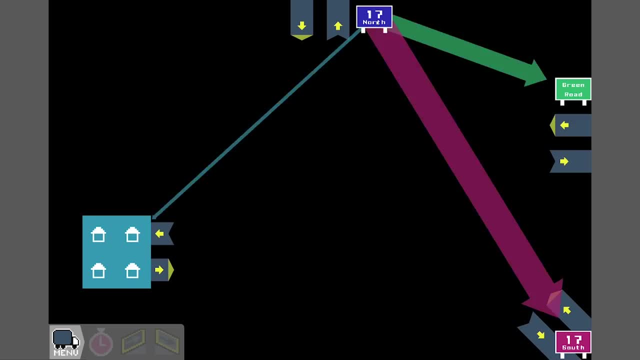 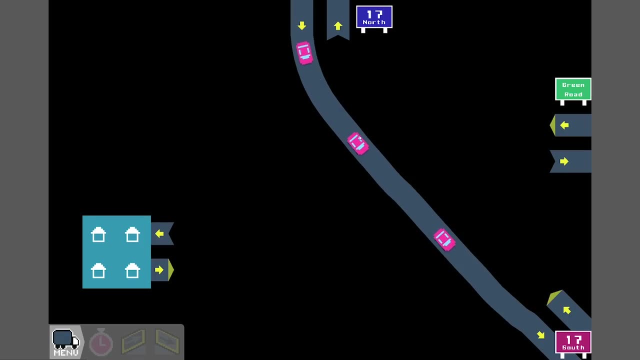 main traffic is going to go. So we're looking here. Most traffic is going to be pink. So as a starter that's going to be your straight through road And the next one is green. So maybe we just want to do simple junction off there And that's green sorted. Then there's a little bit of light blue down. 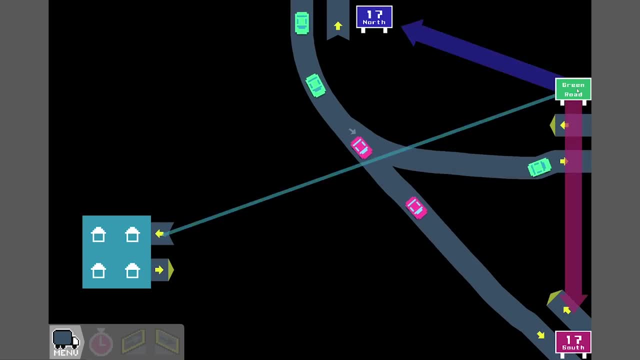 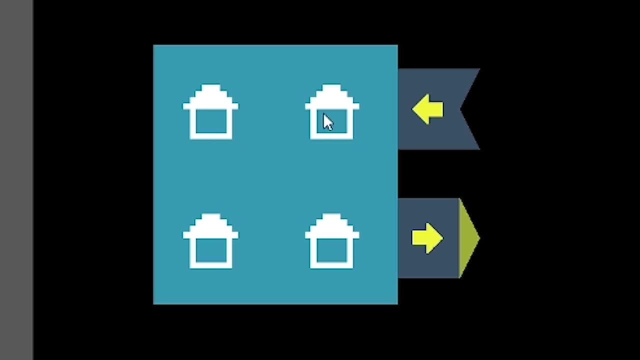 there. We might leave that for now. Let's sort of work out what our next main ones are. So this one is going up to dark blue and down to pink And then a little bit over to there, Which I assume is like some sort of housing estate or something. They look like little houses, Monopoly houses. 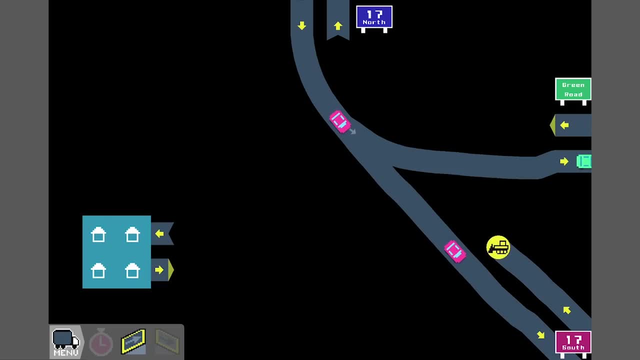 Yeah, and this one is straight up to blue, So I'm going to do the straight up to blue first, So we'll come over here. Now we've got a bridge over that junction. we did Back down Lovely, So that's that. 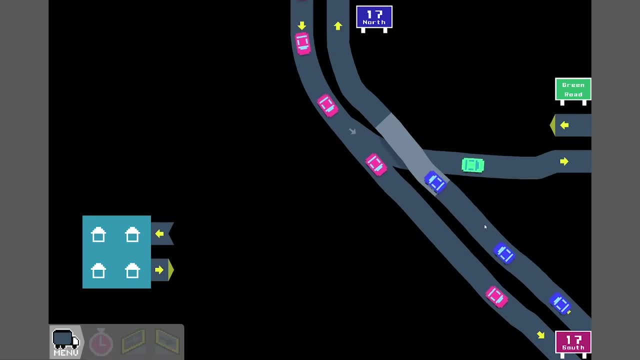 one sorted Right. So now the dark blues want to go to green. So that's a nice easy little shot corner there. Now the one thing I haven't worked out is like: do cars prefer sort of leaving one side or the other? I'm not sure, But I feel like this one is going to be a little bit more. 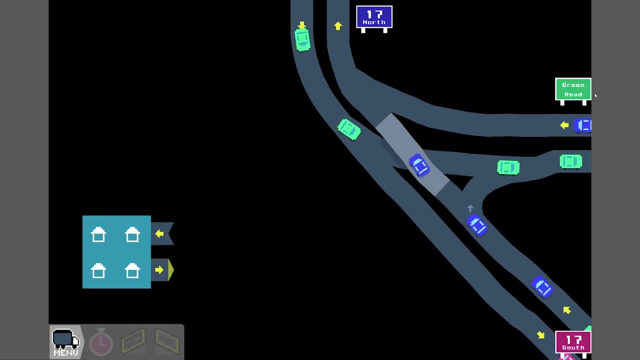 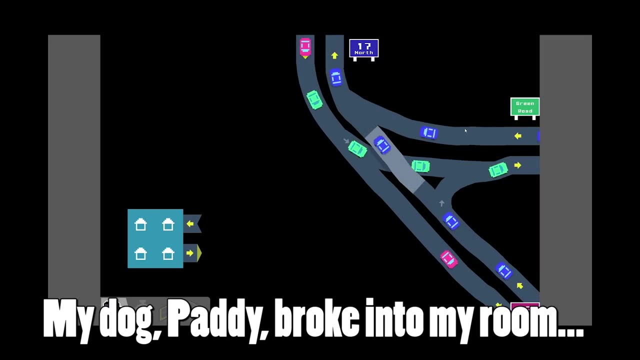 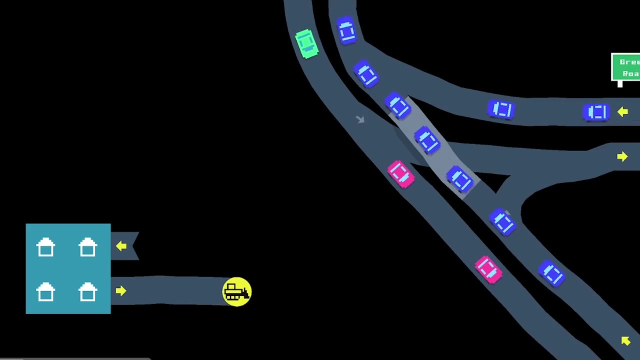 we can just connect on to there, So that green one's done pretty easily. That's busted in, He's busted through the door, He's a dog. He's a dog, He's gone. That's what he wanted to do. Alright, so from this housing estate- Which I think that's what it is- We're 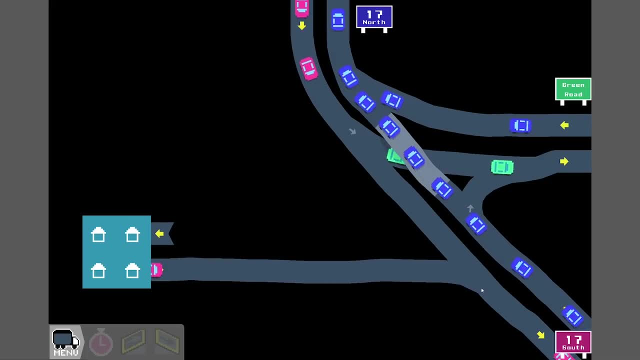 going to come along here Just as straight as we can And just connect in like that. From the blue we're going to come straight down and connect in, like that. I think from this area we come off here. Oh no, I went the wrong way. I went the wrong way. We got a random hill connecting like 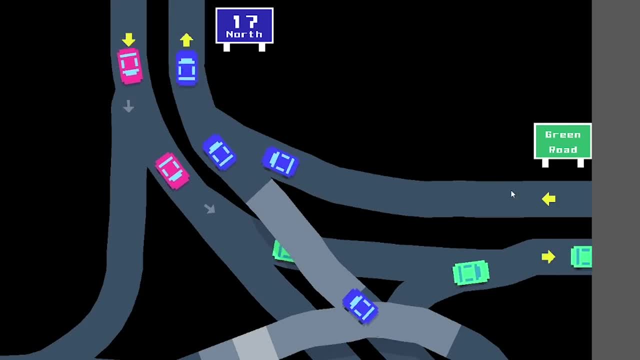 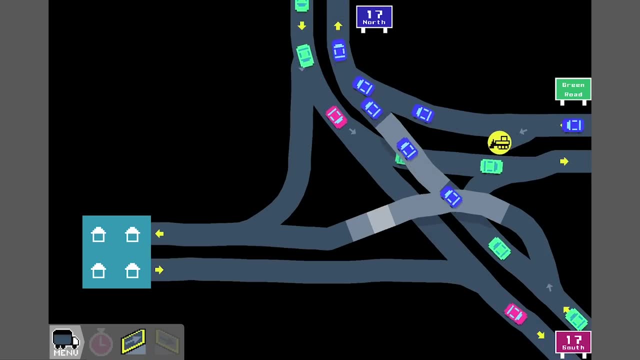 that That's terrible. And then from this arm, This is not ideal, But we're going to go. We could actually try something a bit sneaky So we could come off it. I wouldn't recommend this, But you can come off here And then literally just connect into there, So that works. But we've got mingling. 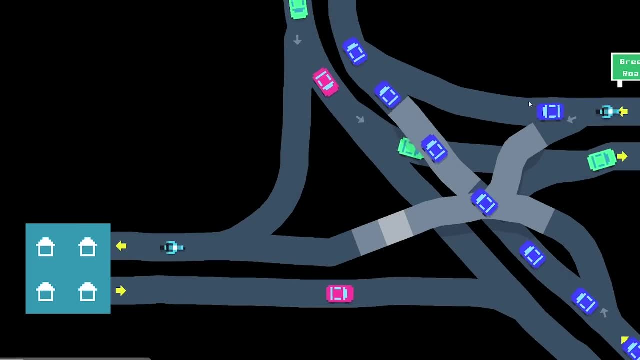 traffic here, But I feel like, as it's so little traffic, Maybe that's fine. I don't know, I might be overthinking, But we're going to come off here with this one as well. We're going to come up and 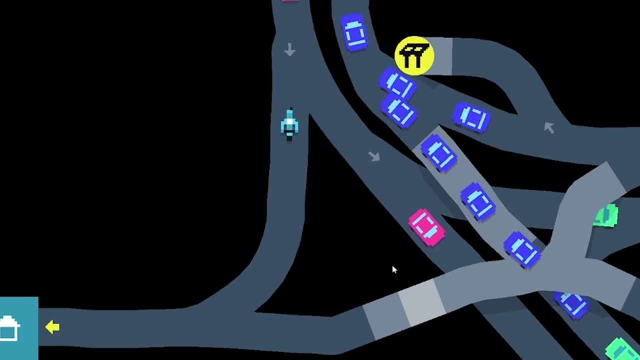 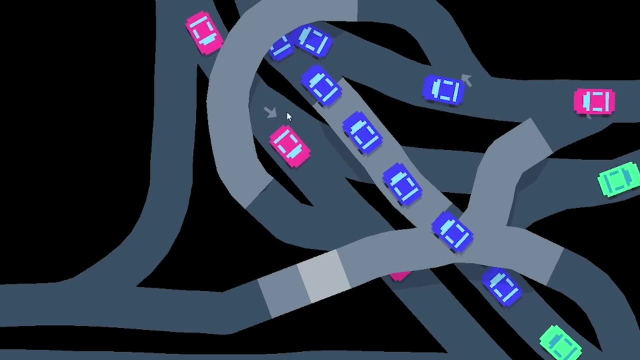 around. We've got to get Down to this pink one And I feel like there's a nice little triangular gap there. Come around like that And then back down And connect in And, if you look, we're connecting in after traffic. 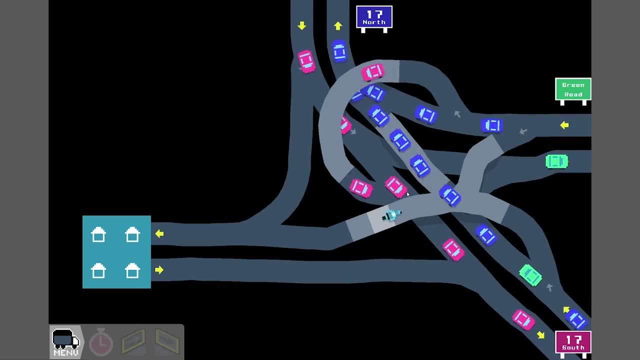 has come off. So you always want to sort of avoid like having a merge on to a road And then off again, Because you're sort of doubling up the traffic. This is ideal, Because you've got people coming off And then coming on afterwards. If it was the other way around, If this We call this- 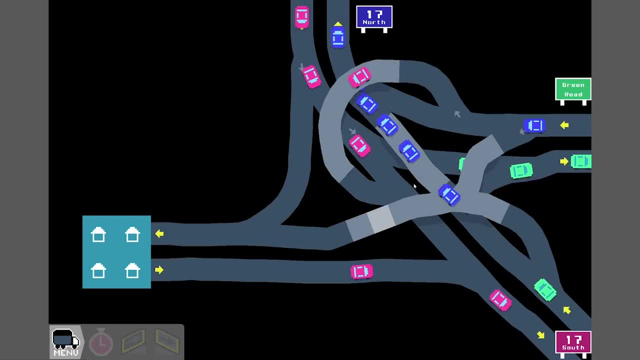 like a merge And that's a diverge. If we had the merge before the diverge, You're like You're mixing up lots of traffic. This, This does look like a mess, But let's see, See how it goes. Oh, we haven't finished, We haven't. 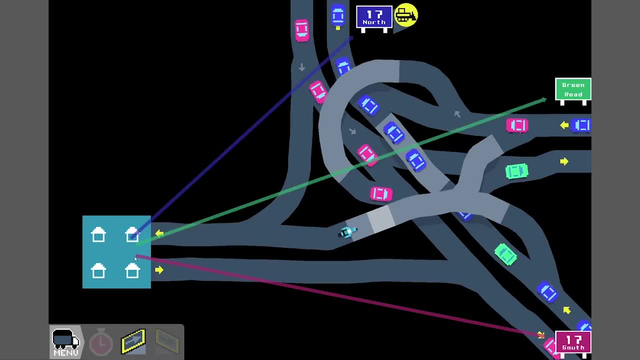 finished. What have we got to do? The game says we haven't finished. None of them are flashing. Oh, do I need to? Oh, we've got to go from here. Yeah, I forgot. I forgot. That was quite silly of me. 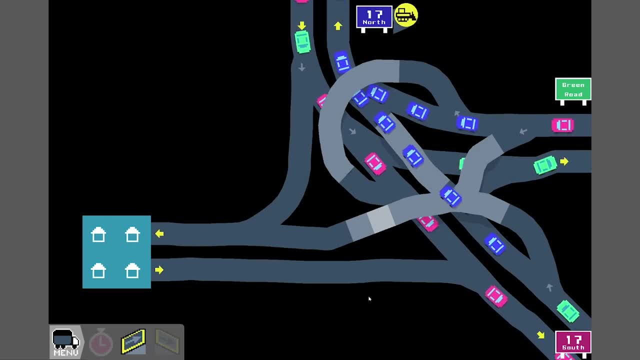 actually Right. So we've got to go from here Over to both of those. Oh, this is getting a bit tricky now, So I reckon we'll come off there, Go up twice. We're over the top of everything. Oh god, My mouse cocked up there- And then we connect in. 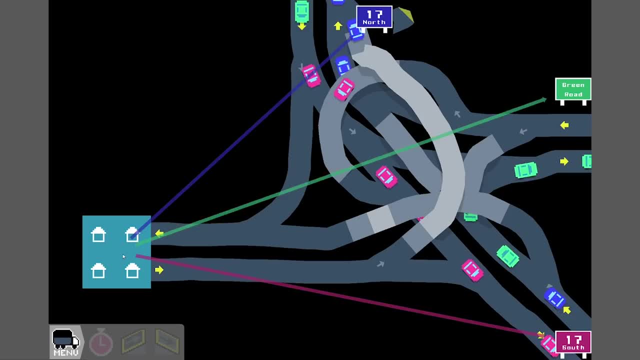 Just about connected in. Look how scraggly that is And, to be honest, it's so little traffic. I'm just going to do a junction from there. I'm going to go down twice Connect in like that. That is disgusting, But it's completed, Let's see how it goes. Look, there's hardly any traffic coming to. 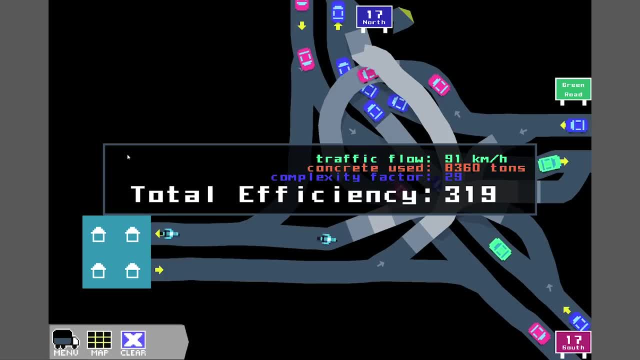 this residential place. So I think that's fine. Total efficiency: 319.. I like that it tells you how much concrete you've used. I feel like that's quite a good thing to try and limit as well. We don't want to like make this super expensive. Look how neat, like the real. 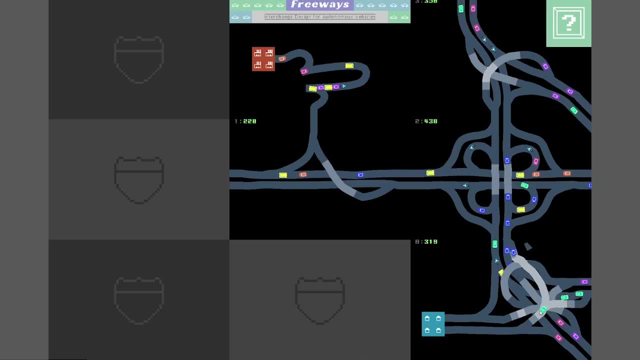 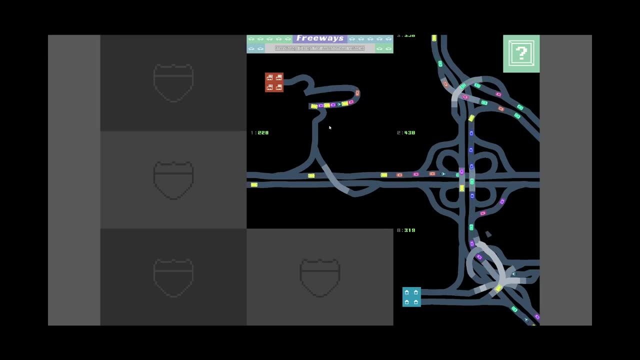 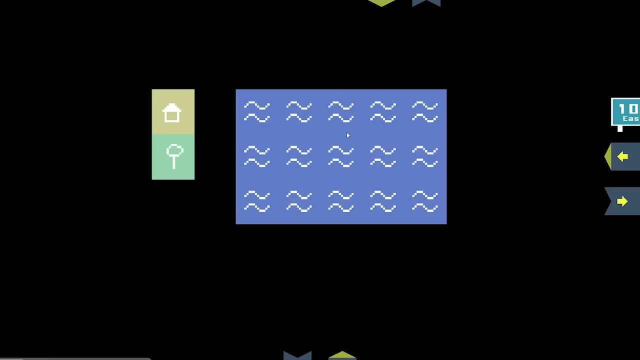 And then just go down the bottom. Oh dear, Oh no, they've blocked up. Look at that, There's a traffic jam. I thought that was the most efficient layout on this thing. I'm going to pick the left one, I think, To keep our motorway running. See where it ends up. Oh, look at this, So I'm not. 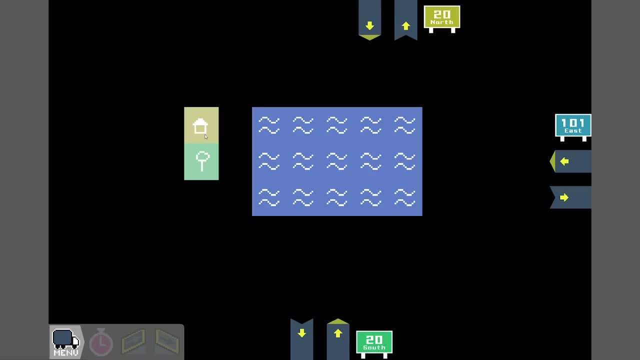 entirely sure what these squares are. It doesn't look like any roads connect to them. Maybe they're just things that you can't drive into, And I guess it's like someone's house and a park or something. But anyway, We've got this water in the way. So if we just have a look at the main sort of direction, It's 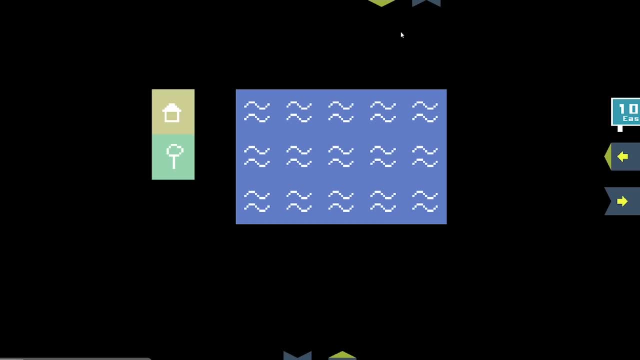 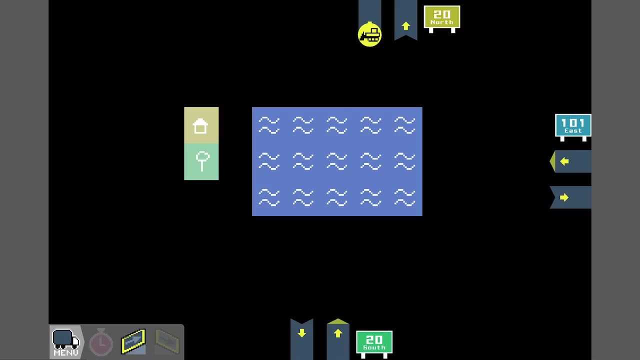 all pretty similar. Right, it's all similar. So for this one I'm going to try and do a realistic one again. It's going to be a bit dodgy Because we've got to think about whether we've got enough height with the water in the way, But essentially we're going to do these as the straight through Back. 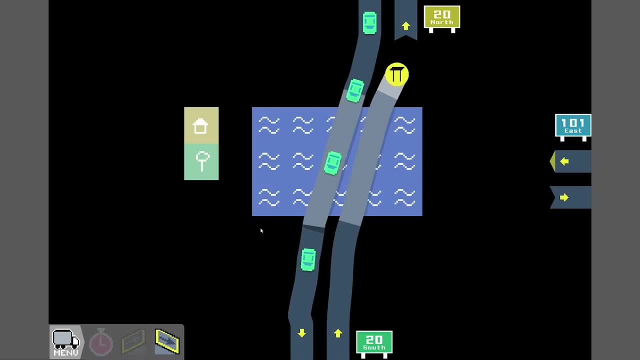 down again. Connect that end Over there Back down. Oh no, I went the wrong way. I went the wrong way. Oh dear, Down Down. Look at that. I wish there was an undo button in this game. I really, really do, So this one's going to be called. 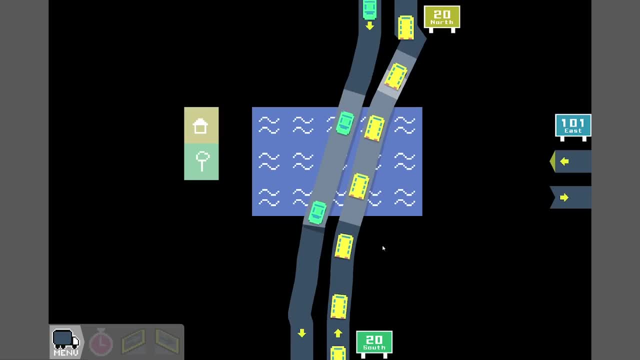 a trumpet, And that's because it sort of looks like a trumpet. Maybe I might actually be able to do this. Maybe we'll get the like photo at the end, But essentially this arm goes straight into there From the green. they go over like that And now all we need to worry about is getting 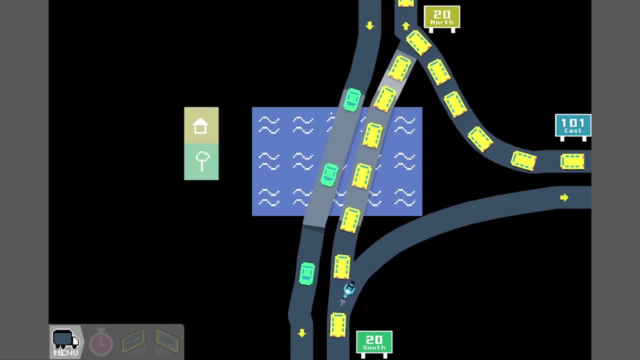 these people onto this road, The green road, And they obviously want to go to the right as well. So for that you take this road, You make it go Straight. We're then going to have to go up- So we've gone over the water- And then to get over. 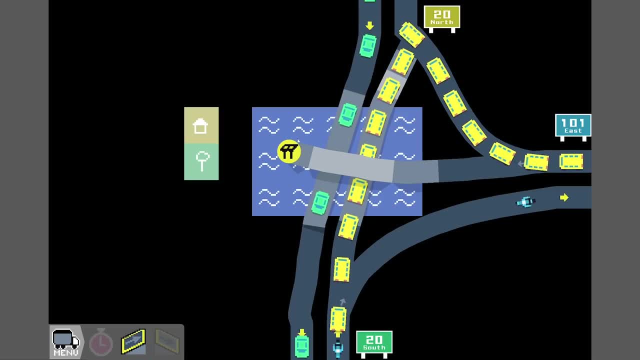 the road. we've got to go up again, So now we can come down. We're still above the water, So we've got to stay as a bridge, But from here we do a sort of round like that, Then we go down And we're. 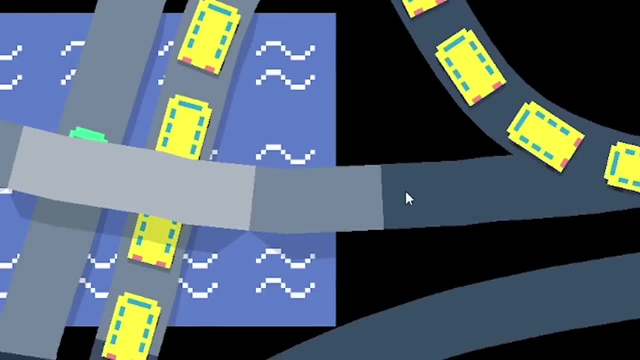 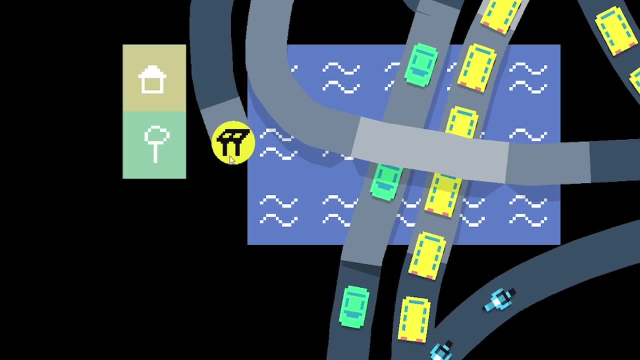 connected in there. So now these people- You can see the green car- They'll be able to come around and go like that. Meanwhile, to get the green cars to go east, We're going to have to come around here And go up over the water And then up over that bridge And then down. 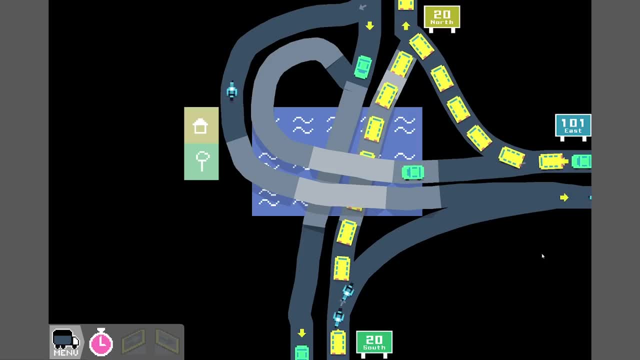 And then down And then network complete And that's called a trumpet design. Unfortunately it's a bit rickety, It's a bit wobbly, But if we simulate this It might show us. I think it did the pick thing after the simulation. No, it doesn't believe us this time, I think because we cocked up. 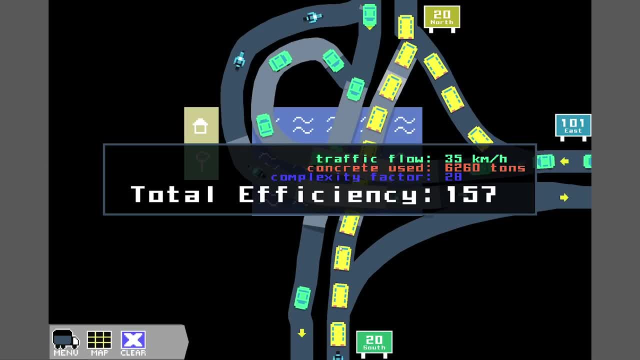 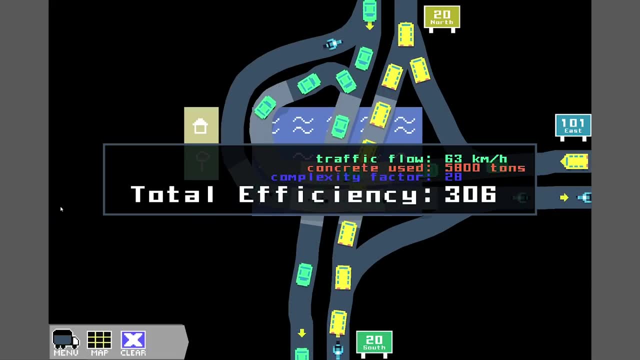 these junctions. So I might just build it again quickly See if having a steady hand will do it any quicker. Is that better? I don't know, This game's hard to draw. My mouse drawing skills are pretty poor. I think efficiency went up though. So sweet, We'll take that No picture anyway. So 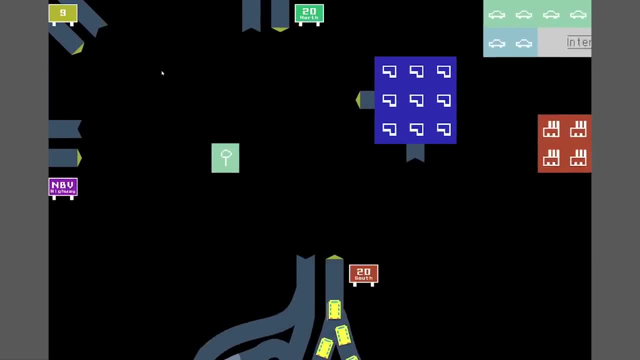 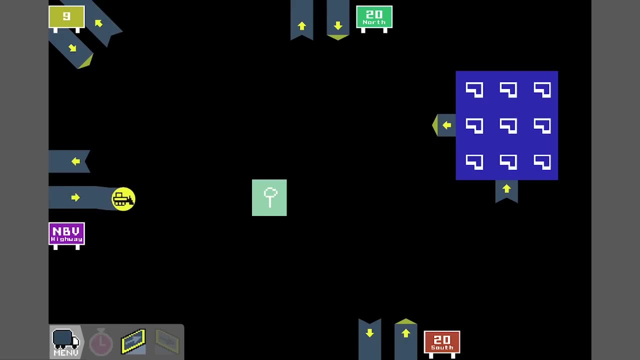 we'll just have to take my word for it. Let's see where all these people are going. Oh god, This looks mental Alright. so I think this one we just free hand again. I'm going to find out the hard way What happens if we go into this. Nope, Okay, we can't go into it. Can we go over it? 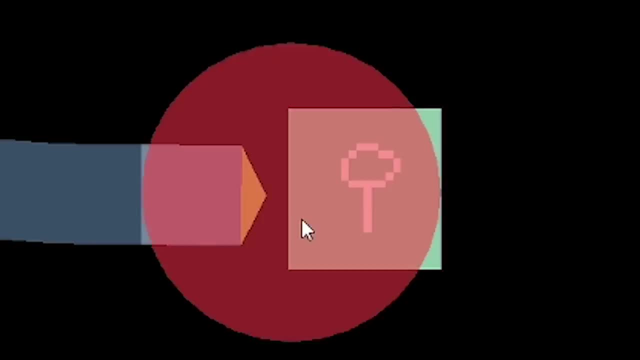 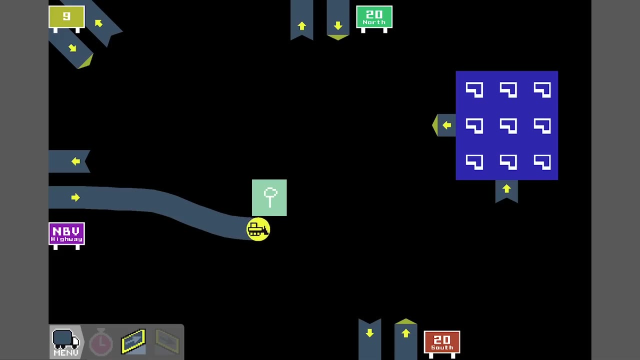 Nope, Doesn't look like it. Can we go double over it? Nope, No. Okay, so trees have to be completely avoided, In which case we'll come like an S bend around there And then we'll do a turn down to there, Because that's the main. 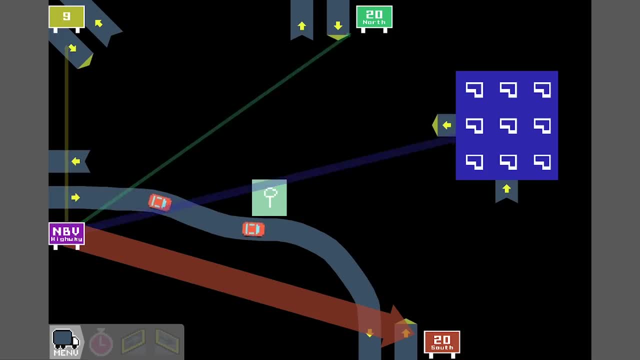 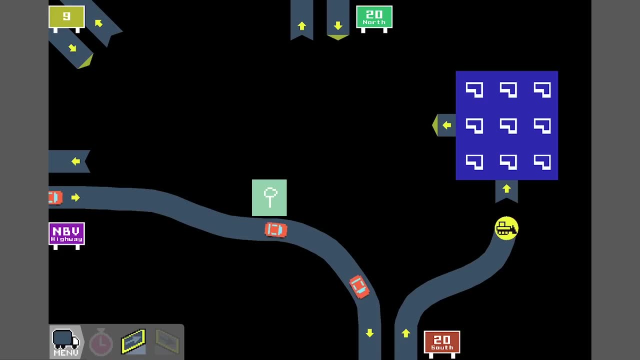 route. Can you see how thick the red arrow is compared to all the others? This one wants to go to the blue, So I think we'll just do like an S bend. So that's those guys sorted. These want to go to the green And greens want to go up there. So I'm going to say I feel like that's like a gun. 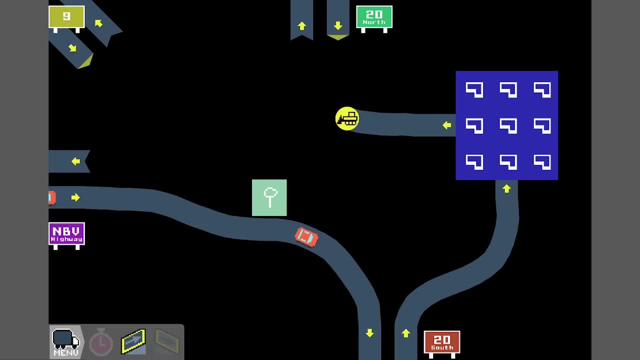 shop Like they're selling lots of guns in there. I'm going to go from the gun shop straight up. This green one is going to be Up and over Like that. This one just wants to go down there. So that's pretty simple. 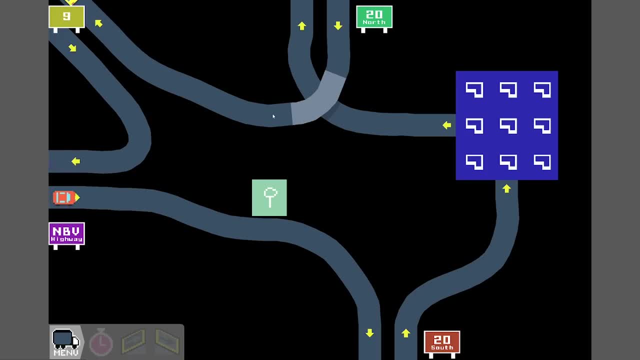 Annoyingly. I could have done some way more sensible stuff If I'd made that bridge slightly longer. I could have taken these guys underneath, But I guess I could just do that And connect before it. I can also bring these guys onto the reds before the tree. I could do a junction off. 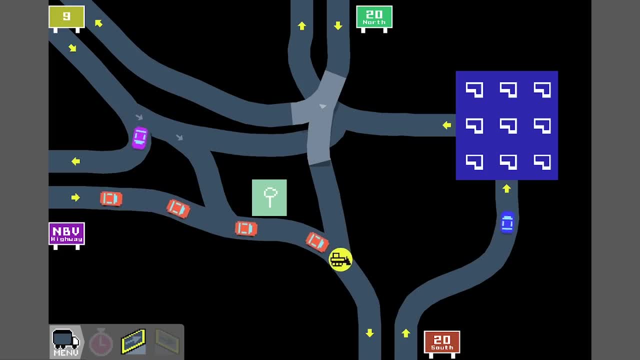 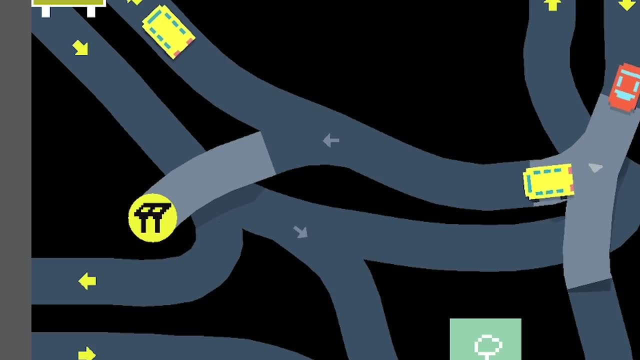 the bridge And then down, And that can go straight onto red, But it can also swing around for the blues as well, And then we can come off on the left side here Over that Back down Onto there. Just nice little Little bridges Everywhere. So I think that's all those. 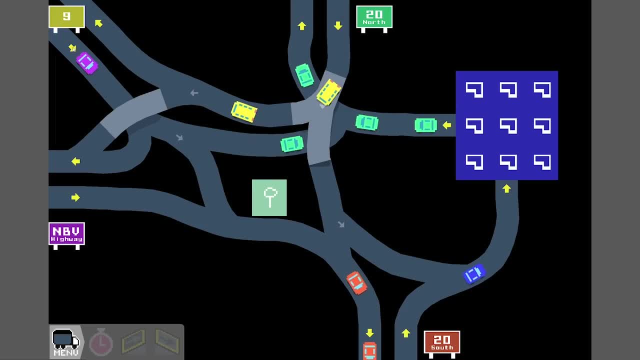 done. Yep, No flashing Yellow, We've just got to get to blue. So yellows come around here As they've gone under that bridge, I can take them off like that, Probably just connect them straight onto this one. This is looking a mess. I probably should have done like a roundabout, for 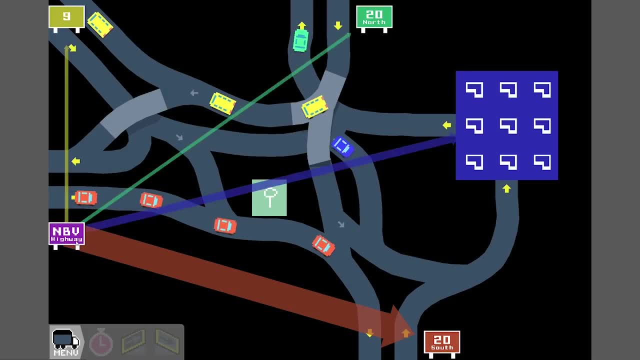 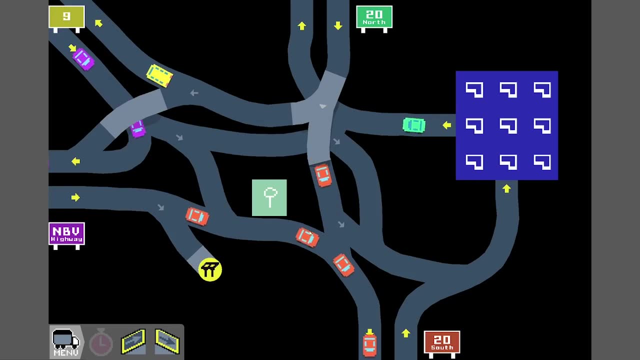 this. I wonder if you can do roundabouts in this game, Right? So purple wants to get everywhere, So I'll probably take them off before these guys merge. So you're coming off here. I sort of feel like a loop round to there, And then we can do like slip roads off. So if we do like that And 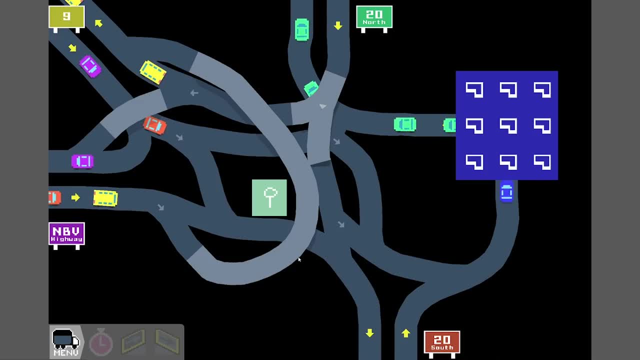 then ideally connect this one after that diverge. So that's that sorted, We can come, We can get them to the gun shop by doing that. That's not ideal. I probably should have tried to connect in a little bit sooner, But oh well, And then again we can come off like there, Come down and 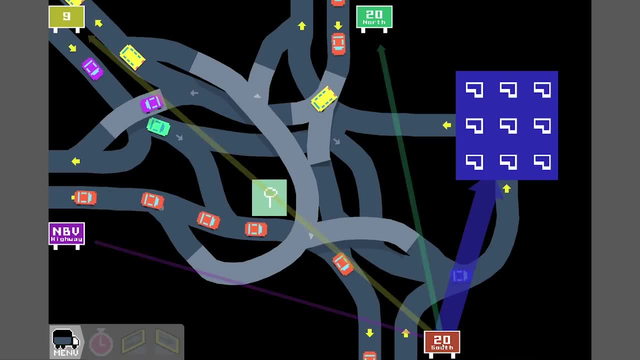 connect in. So I think that's all of those done, Yep. And then just from 20 south, We've got to go every direction possible. So with the mergers there, I want to take these off Four. pretty much, We'll come off, We'll go. I think we'll do something similar And that will come. 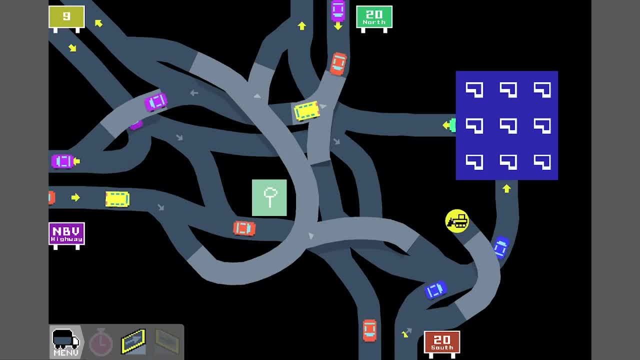 up. I'll try and limit the roads. I don't want to do like a massive overpass, like that. We'll come along there And then we'll have to go up over that And we'll have to go up again to get over. 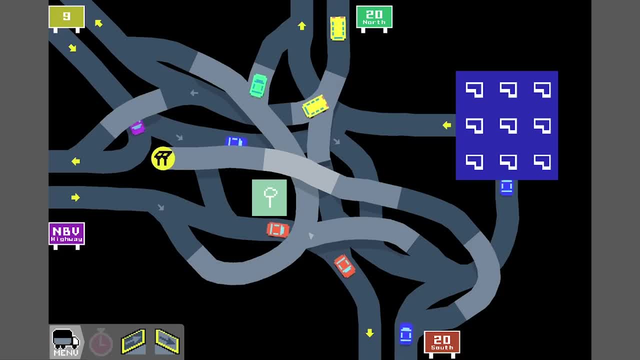 that one, Yeah, But then we can come down once And I feel like straight into there will be good. So down Connected in Lovely jubbly. To get to the green, I'm just going to join the gun shop. yellow. I might just say: let's connect to this bridge. So we've got. we got a diverge there. So if 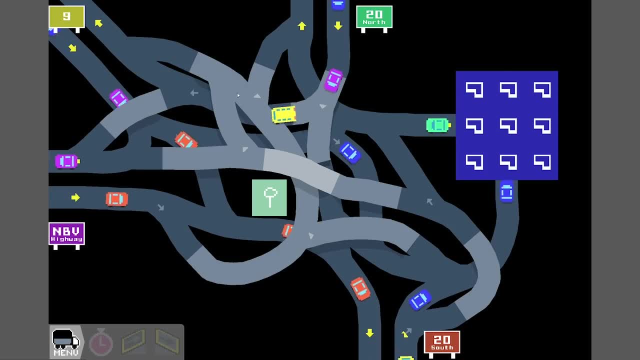 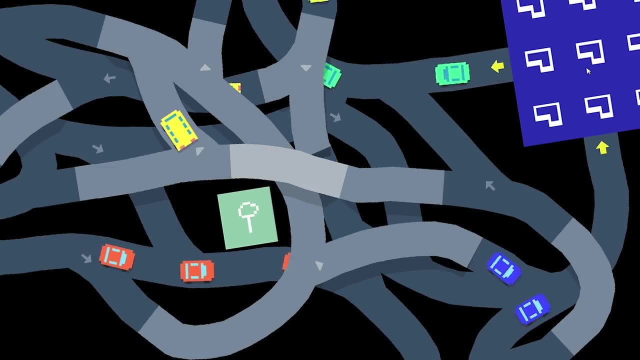 we come off there, We can connect just off the diverge And that's everything done. No, it's not everything done. We've got it. Oh god, this is so complicated. I have proper messes up. So we're going from the gun shop. We've got to get to all the routes, So I'm gonna. I should have just done. 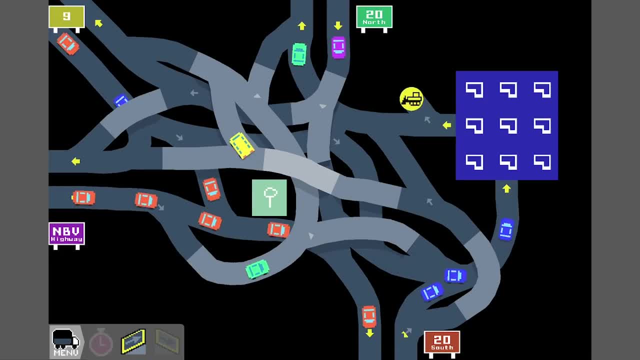 a roundabout. I really should have done a roundabout So for this one. then we're going to come out And I'm literally just going to do a massive loop, Round the entire of everything. So around that, Around, that, Around that, Come down here And 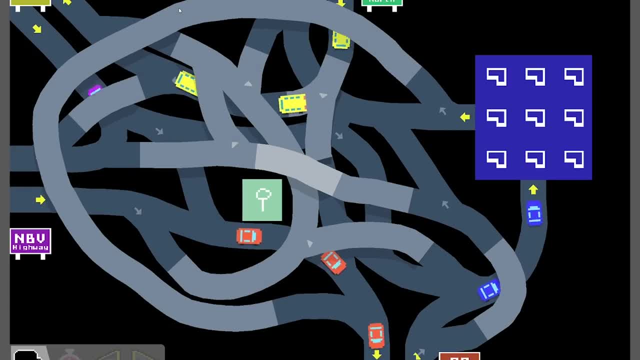 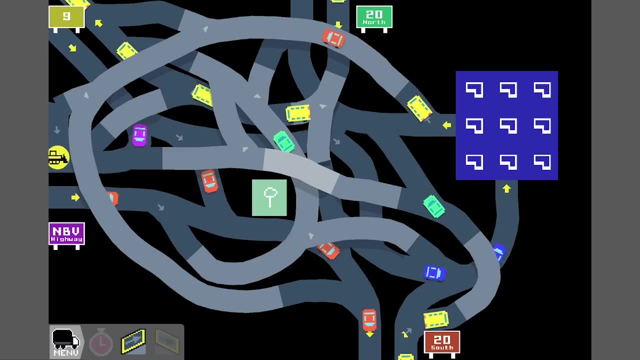 connect into that. Then if we want to, What is this? So, if we want to go yellow, We come off And then go down. And then if we want to go purple, We do the same: We come off And then we go down. 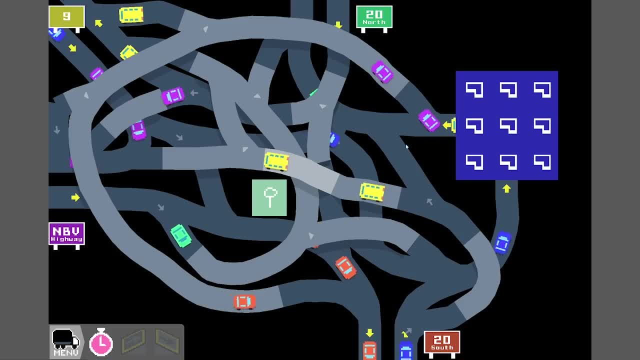 Network complete. This is also a realistic one. I like to call it the brain, Because it looks like a brain. Oh man, What a mess. Let's simulate this. Seems to run quite smoothly, though I'm not seeing anything back up too much, But uh, 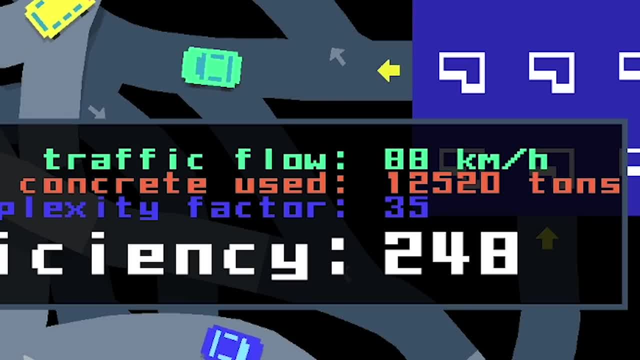 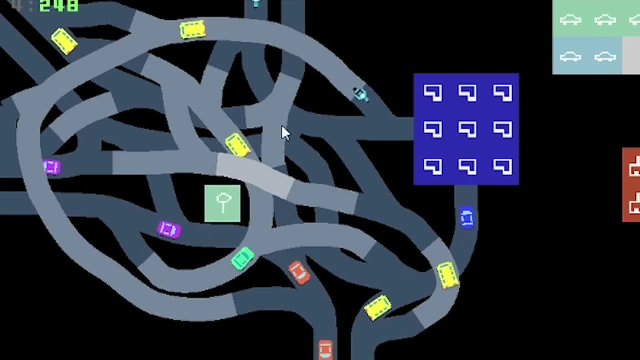 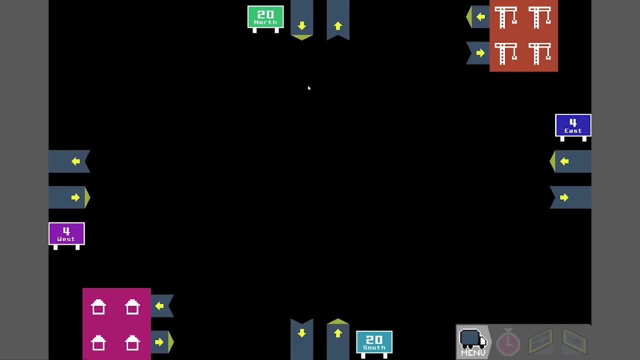 Look, Look how much concrete we used: 12,520 tons of concrete. That's a lot of concrete. I love how simple it started And how complicated it's gotten. Let's have a go at this. I'm right for this one, Sod anything. I'm just going to try and do a roundabout. This is going to be like. 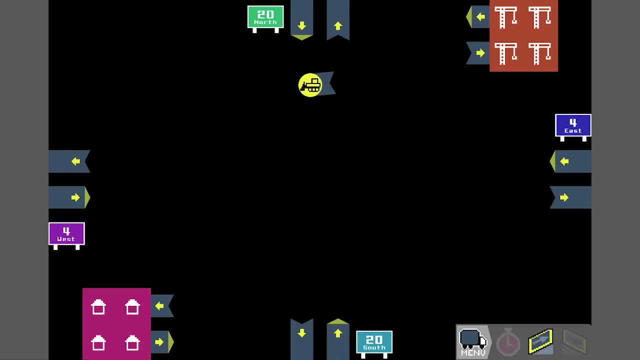 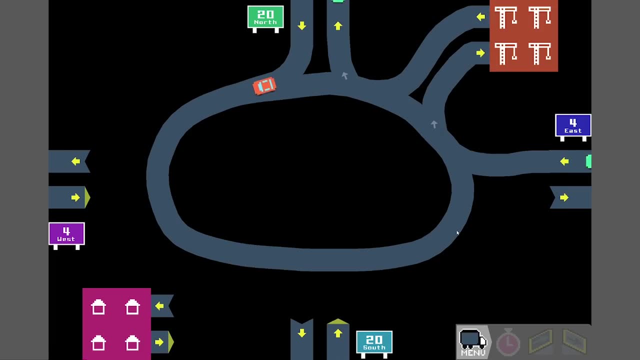 a crazy ass roundabout. So I'm literally just going to do big as possible Like that, And then it's pretty simple. We just do an on And an off And an on And an off, On Off, On. 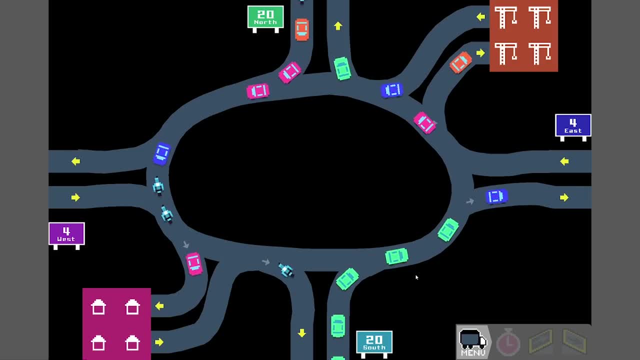 Off. Are you seeing a pattern Right? So that's all journeys complete. There is actually something else you can do with roundabouts to make them a bit better. They're called like hamburger roundabouts And essentially, if we, If we try and find like one, that's got a really Yeah. So 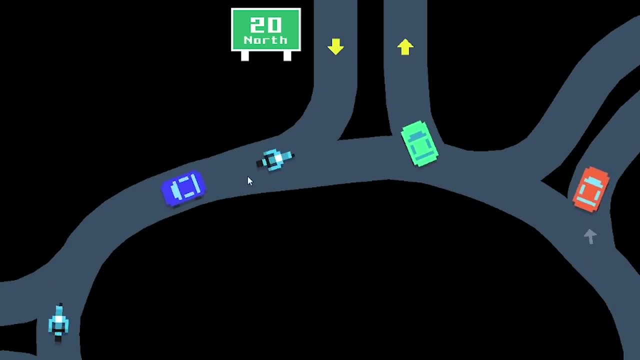 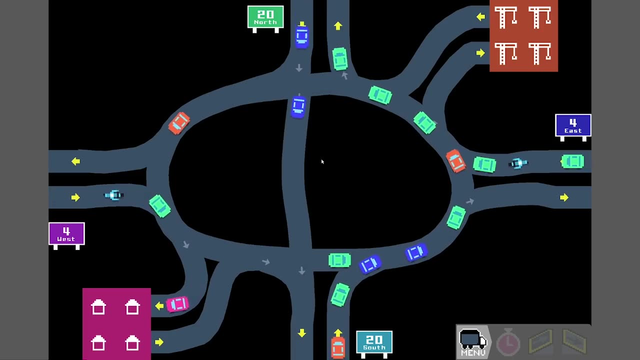 green really wants to go straight down, So it seems pointless to bring these guys all the way around. What we can do, We can make a hamburger Which essentially does that. So it's like a straight through And now you can see. if you turn your head, This now looks like a burger As this: 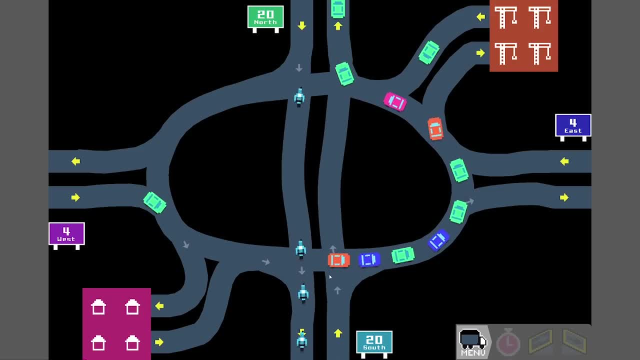 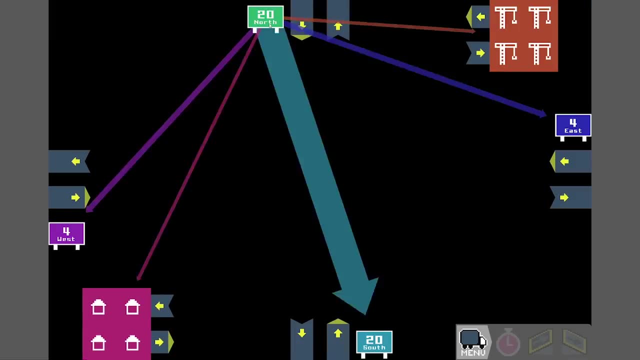 one is the same. We can just do that, and generally these are like signalized, so you'd have like traffic lights and stuff. but that should be working and it's not. so i don't understand why it's not okay. fine, let's clear. now we have the knowledge. i probably should have checked the signs first. it looks like everything's. 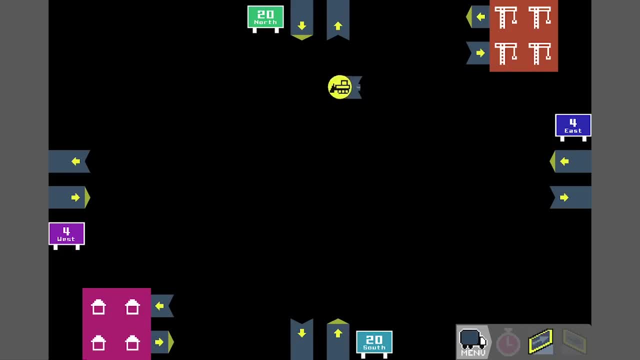 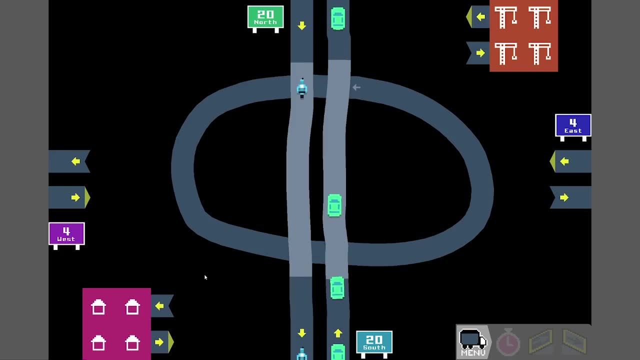 pretty small apart from the main route. i do want the roundabout to work, though, so let's draw the roundabout back in, but this time we'll try and do the straight throughs, and then shall we just try and round about everything else, or should i try and i can do straight throughs, like with the blues? 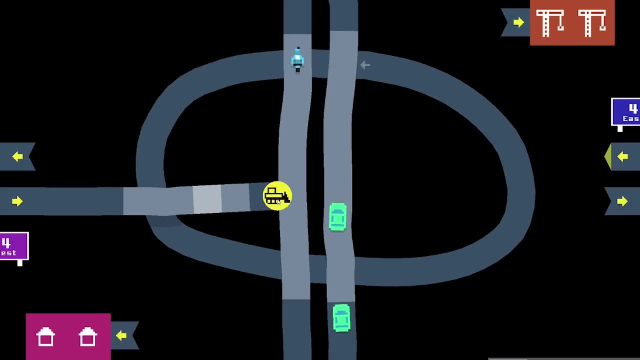 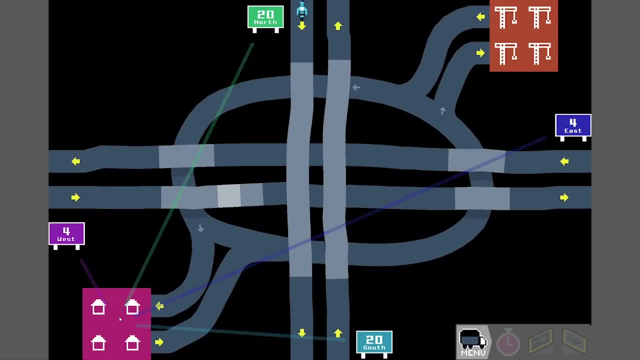 so i can just go over that. oh, bollocks, wrong way, wrong button. i always get the button wrong. do that? come over there, come down under that, up over down connect. oh, i've just noticed, actually these don't go to each other, they're just destinations. ah no, there you go, we've done. 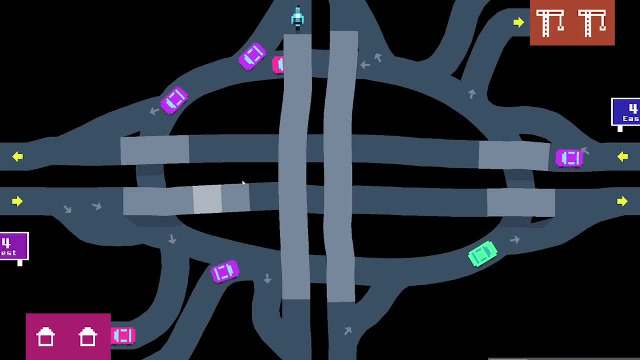 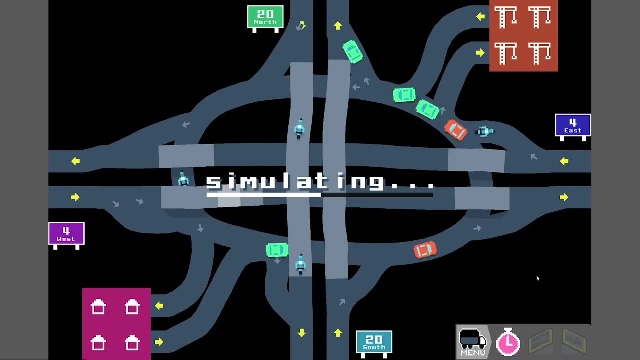 our crazy roundabout hamburger thing. it's more of like a jacket potato. now it's cut in a cross section, but let's run the simulation and see how efficient it is. it's looking good, you can see. there's way more traffic going through here and there's a lot of traffic going through here. 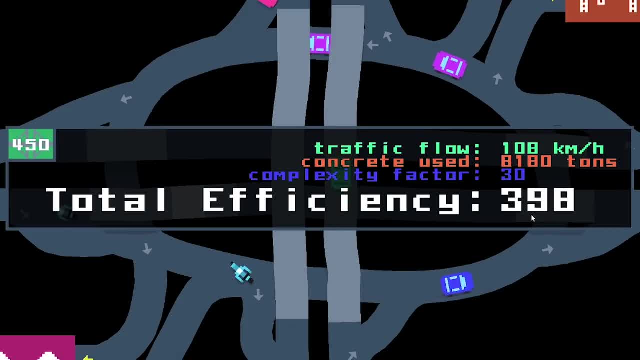 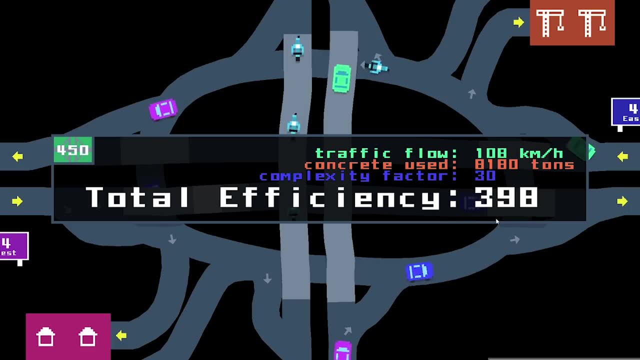 vertically. so that's why we split that up. oh, that's not bad. nearly 400 efficiency. i feel like that's sort of like how you know you're doing well. i think in the 400s you're doing good. you're over 300. maybe you're getting there. if you're sort of under 300, i think your road needs a bit of work. 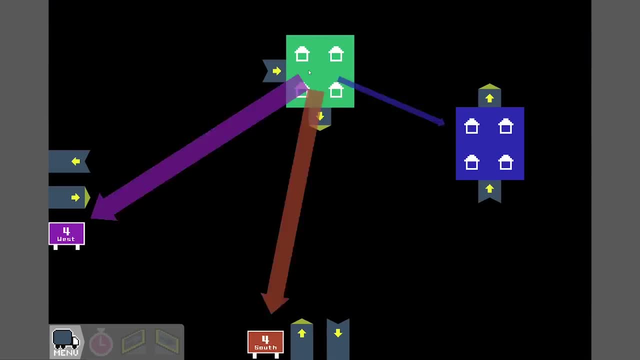 but yeah, that works. now we'll have a look at this one in the middle. so, looking at these, we've got to go everywhere. yeah, we've got to go everywhere. and they're all pretty, even like all the arrows are the same thickness. so i think, to start, i want to probably just put a bend in like that for that one. 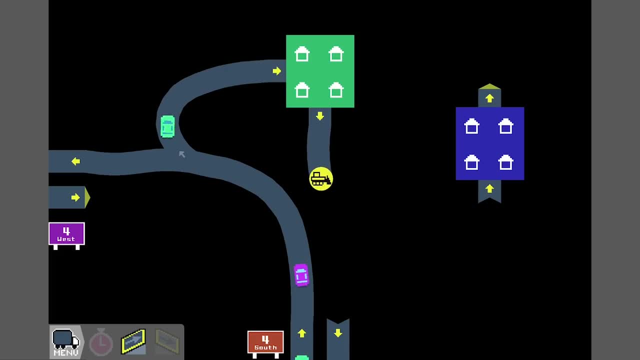 then maybe come off there for that one, for this green, i'll just go straight down. it's a little bit wiggly again, damn wiggles. it's this one. we're going to come straight and we're going to go up and over and then come back down and connect that in there. take that one around like that, meanwhile coming. 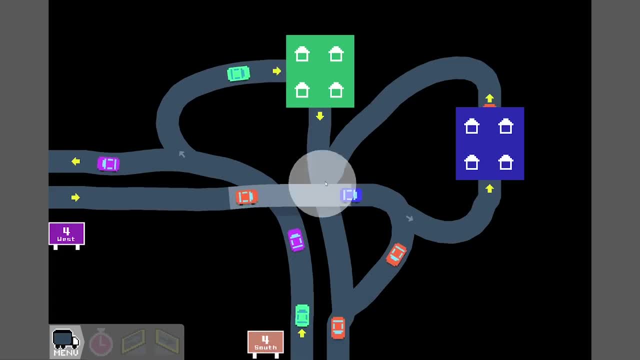 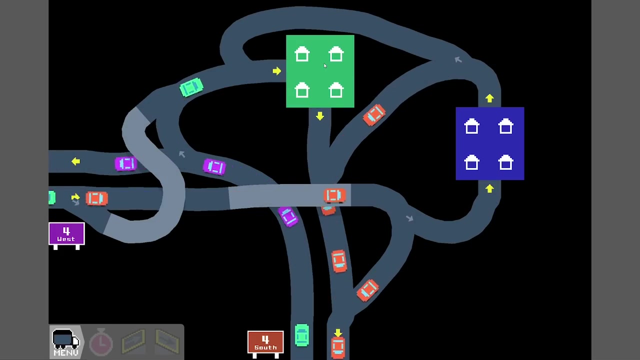 out of the blues, come around and connect to green before the bridge. you can also come off there and do a little sweepy turn like that. you want to come off here, go up and down like that stupid ass bend. you'd never do an s bend like that, but we have. but we have out of here, we'll just connect that. 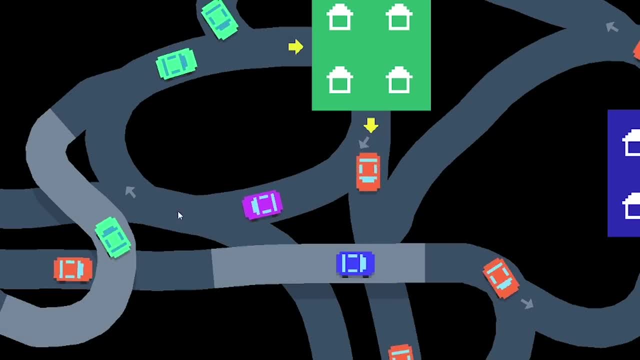 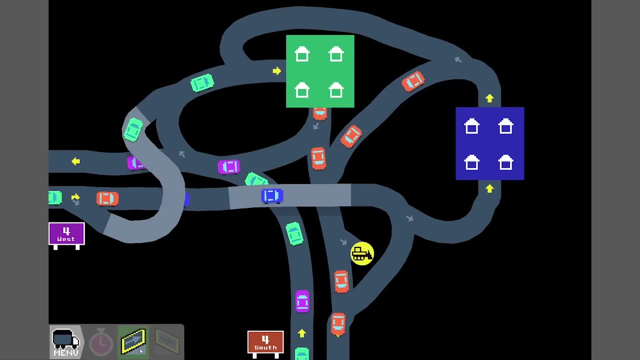 way again. that's not ideal, because you've got a merge and then a diverge, so this stretch of road will get busy and then i probably could have done this better. but we can take these guys off, go over that road back down and connect in. is that everything done? no, not quite, because now we need 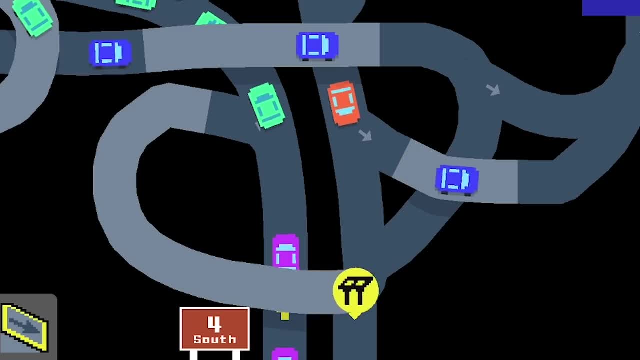 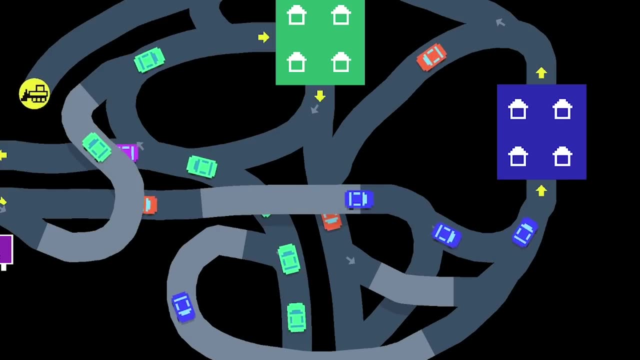 to take you. oh, we didn't, we didn't need to go up at all there until there. bring you back down, connect you in and then, finally, from this point on, we're going to go up and connect to green, and then we're going to connect to blue just to get to the purple. we can just come around there. yes, you can tell i'm. 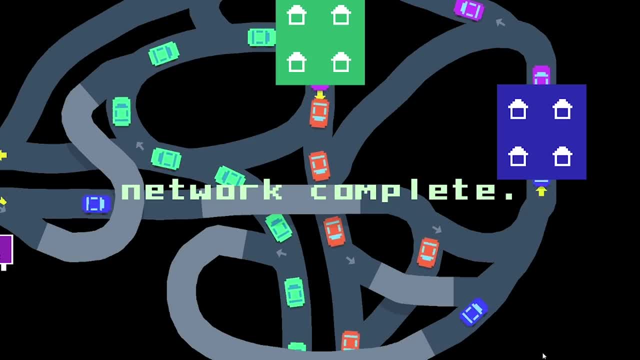 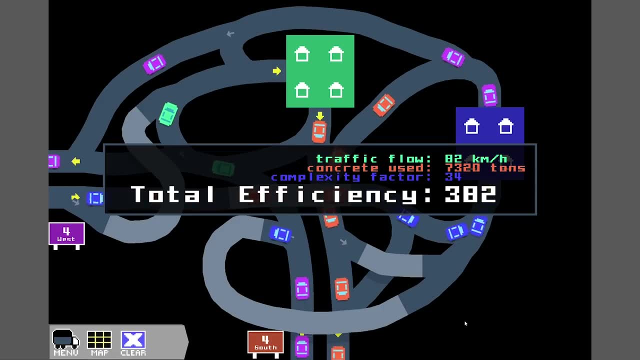 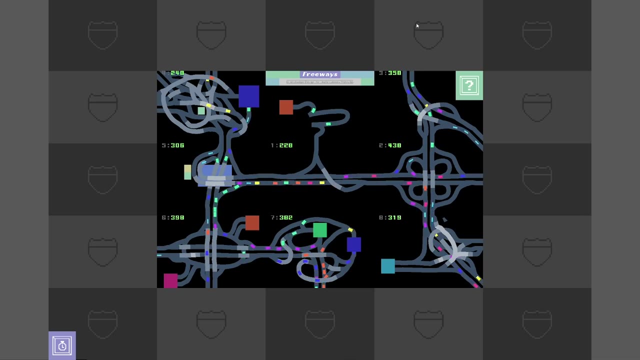 definitely a real highway engineer. look at this. let's simulate anyway. let's see the horrors that i've created in numbers 382, the high 300s. i think i did all right somehow. anyway, we'll go back to the map and now you can see we've expanded, we've got a whole host of new levels at that top left. 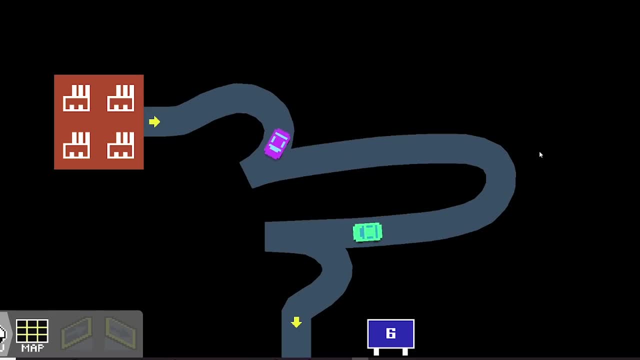 one, and you can see just by looking at the traffic: the most efficient shape clearly is this one. but yeah, that was. that was pretty good. i think i'm going to go back to the map and i'm going to go freeways. i hope you enjoy that, guys. if you enjoyed this, if you want to see more, maybe we could go.